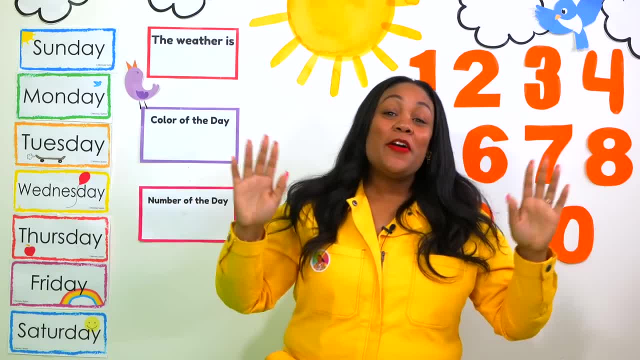 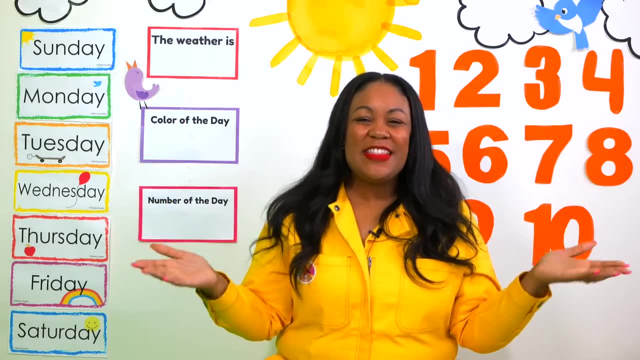 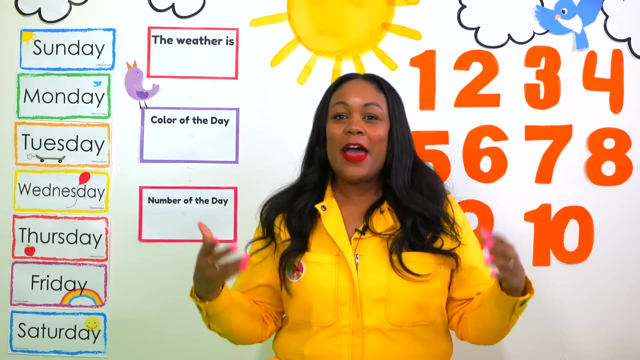 Good morning, good morning. good morning to you, Good morning to everyone. and how do you do? Hello friends, Welcome to the circle time classroom. I am so happy you're here today. Oh, can you give me a big wave? 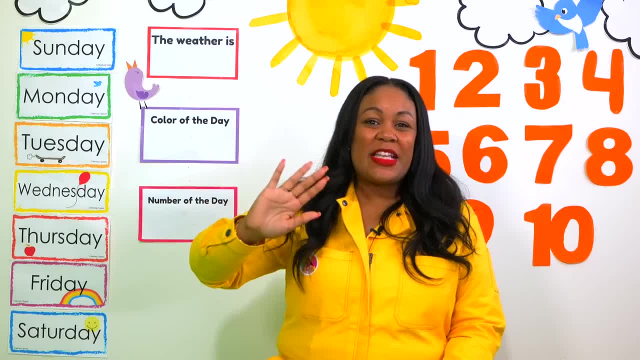 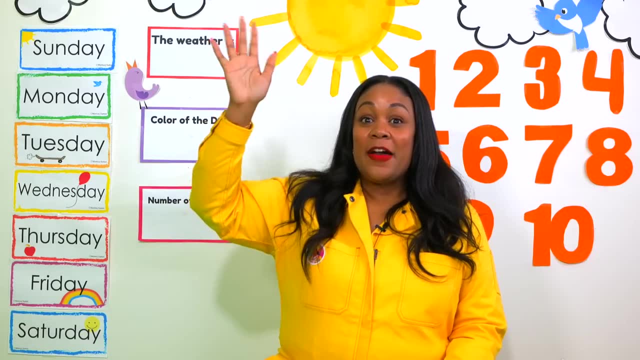 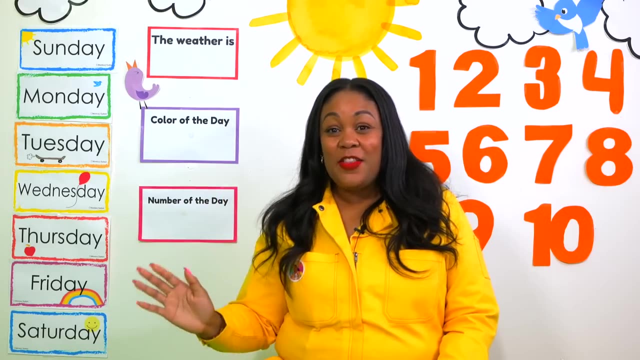 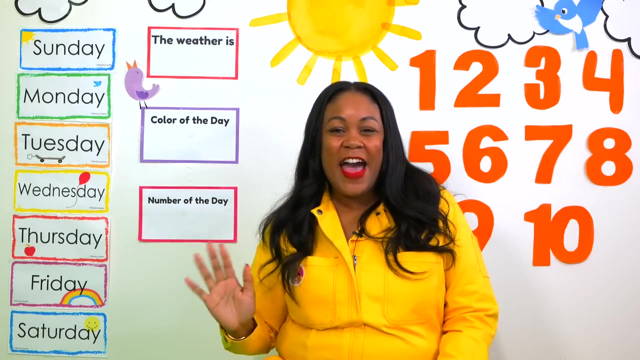 Can you wave your hand? Yes, wave from side to side. Wave from side to side. Can you wave high up high? Can you wave down down low Again? Can you wave high up high? Can you wave down down low? Good waving. 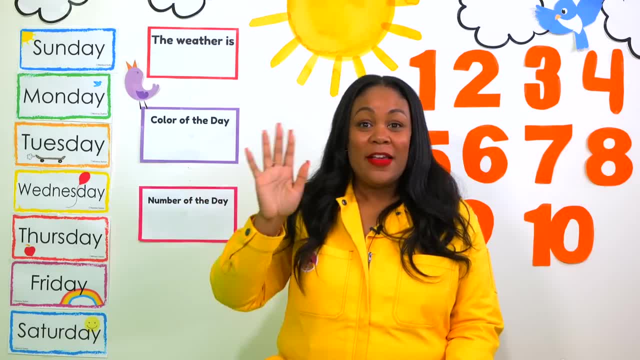 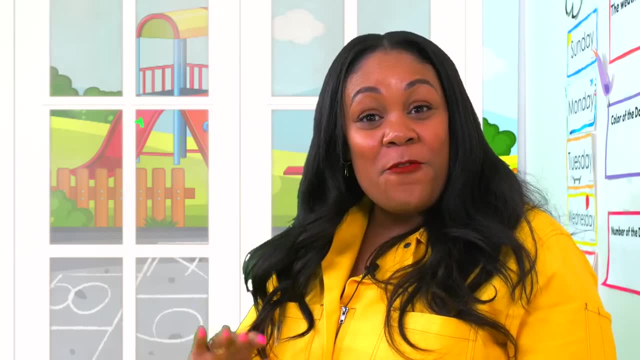 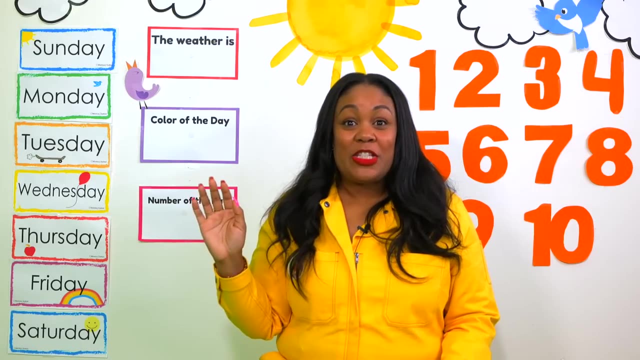 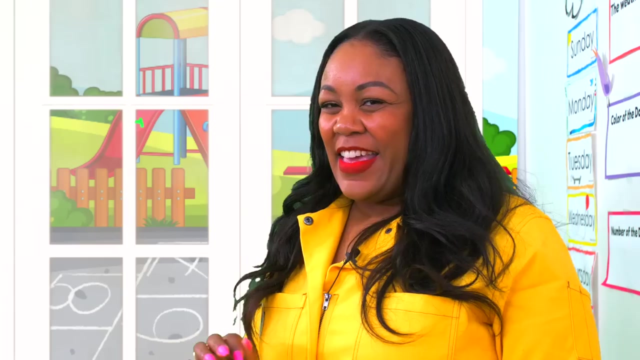 Oh, can you wave slow? Let's try. Can you wave slow, slow, slow, And can you wave fast? Let's try fast, fast, Let's try, slow again. Can you wave slow, slow, slow, And can you wave fast? 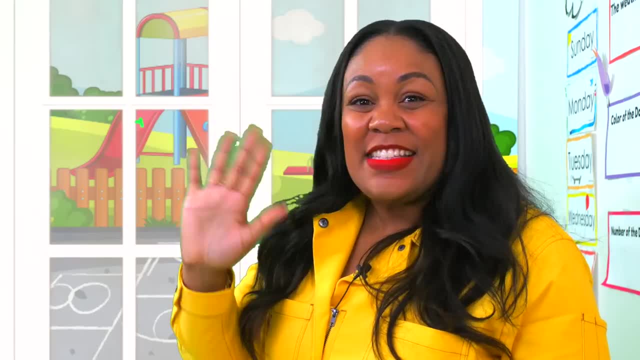 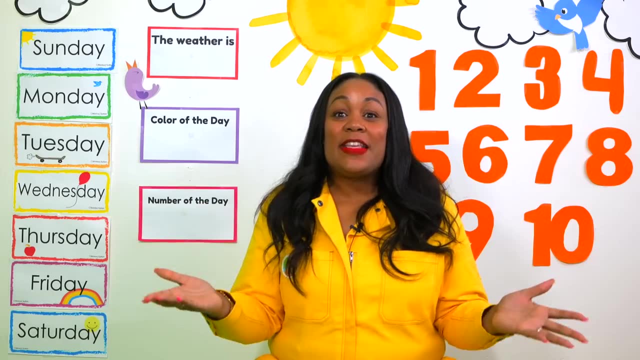 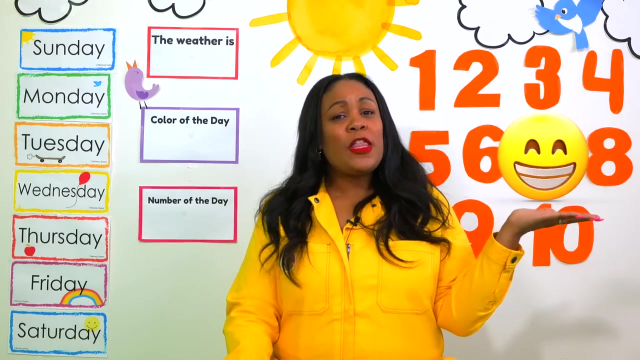 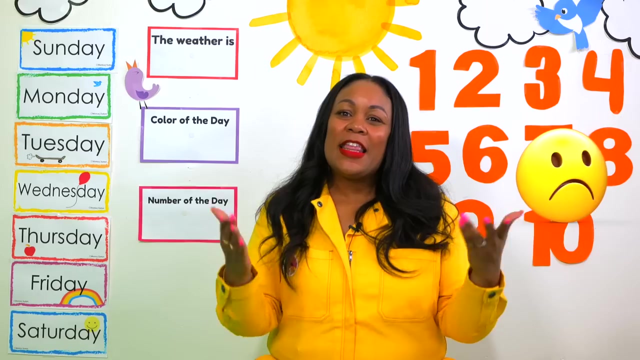 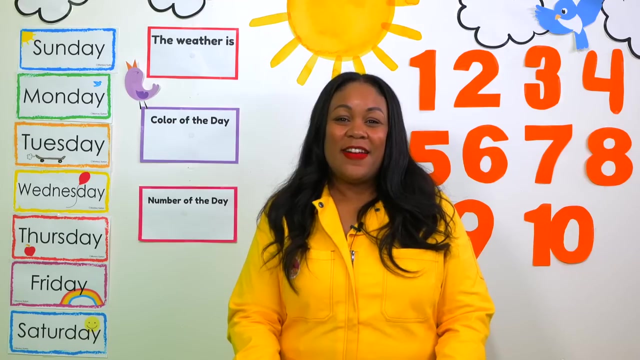 Let's try. Can you wave fast, fast, fast. Oh wonderful waving Friends. how do you feel today? Are you feeling happy Smile, Or are you feeling sad Frown? We all have so many feelings. Will you sing the feeling song with me? Great, Get ready, Get ready. 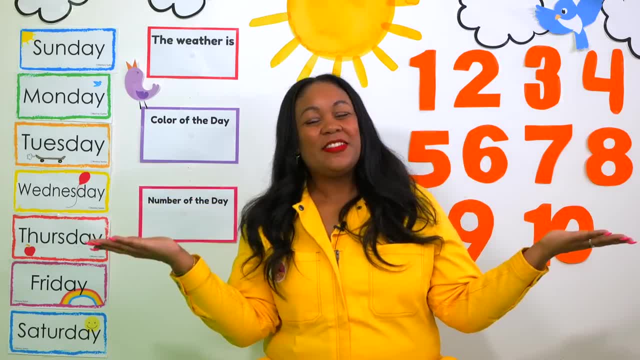 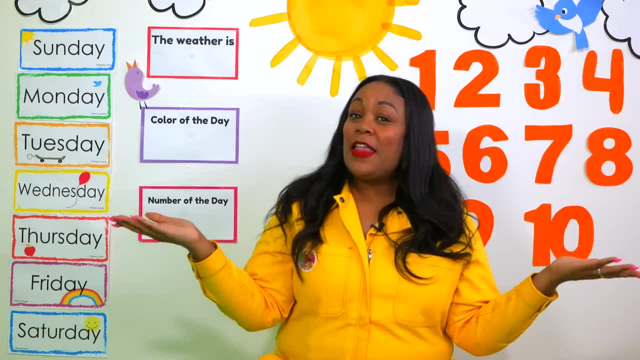 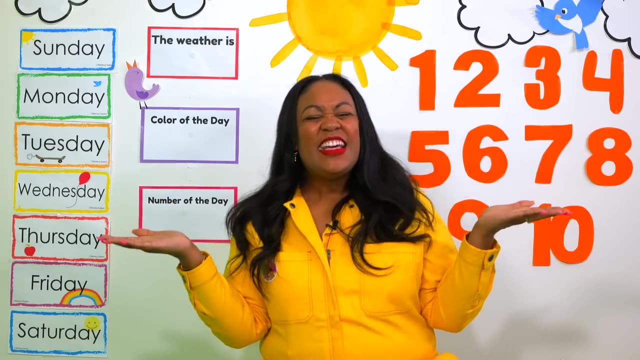 Here we go. I have many feelings. Feelings are what I have. I have many feelings. Feelings are what I have. I have many feelings. Feelings are what I have. Sometimes I'm happy, Sometimes I'm sad, Sometimes I'm silly. 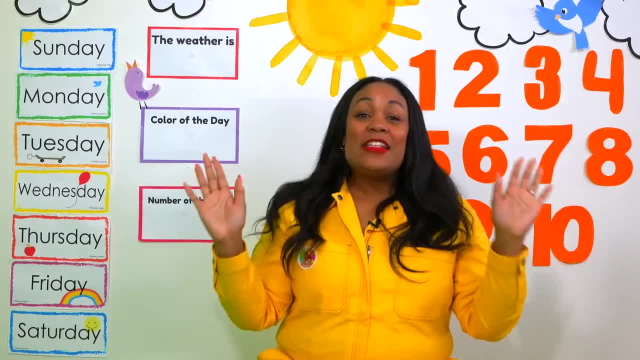 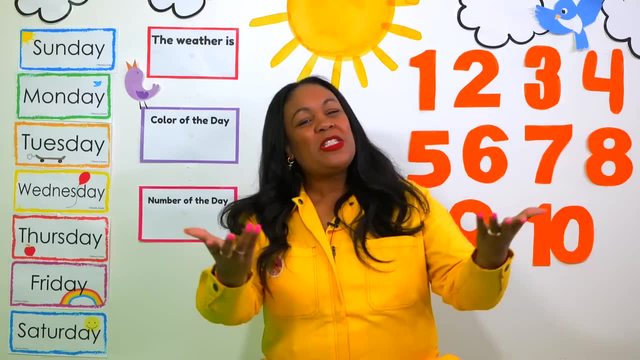 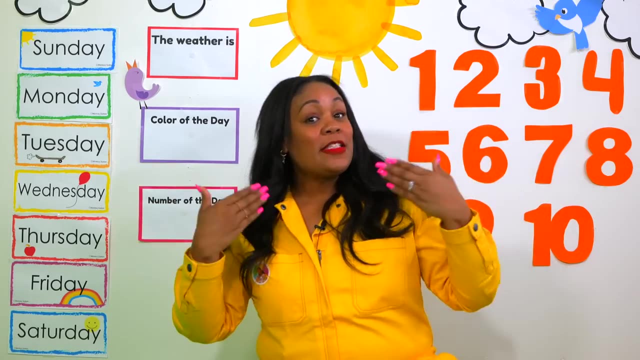 Sometimes I'm mad, Sometimes I'm sleepy, Sometimes surprised. When I'm scared of something, I close my eyes. All these emotions, they can make me cry. I have many feelings. Feelings are what I have. I have many feelings. 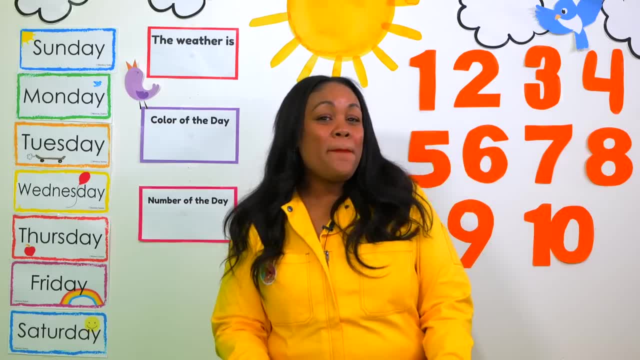 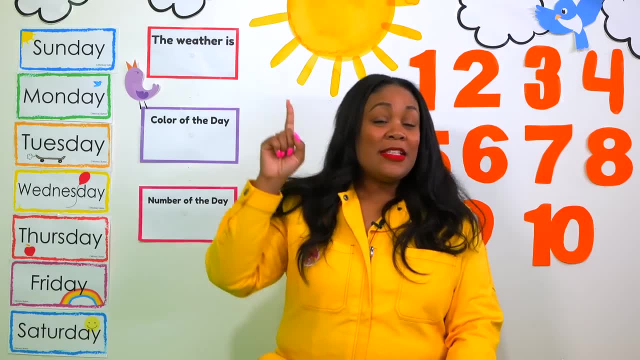 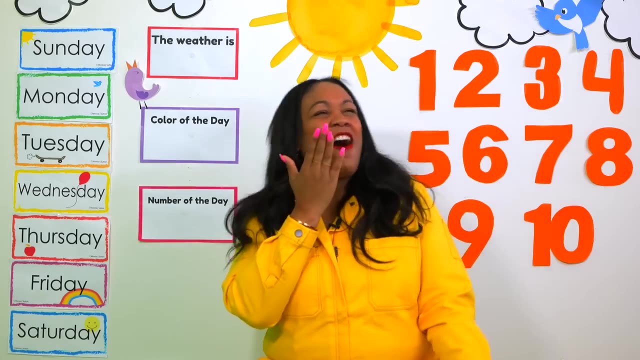 Feelings are what I have. When I'm happy, I like to smile. When I'm sad, I make a frown. Sometimes I'm up, Sometimes I'm down. When I'm silly, I laugh out loud. Now I know. 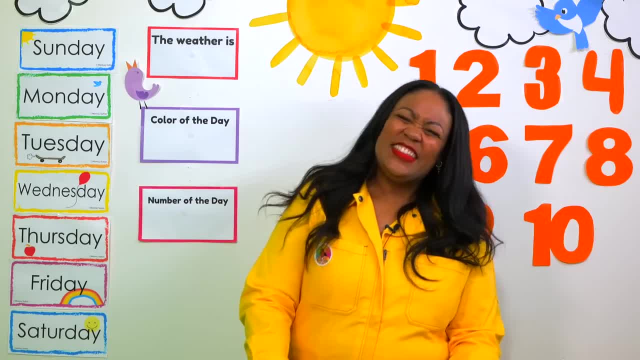 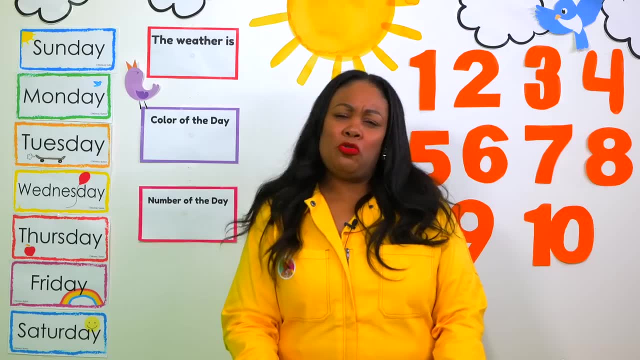 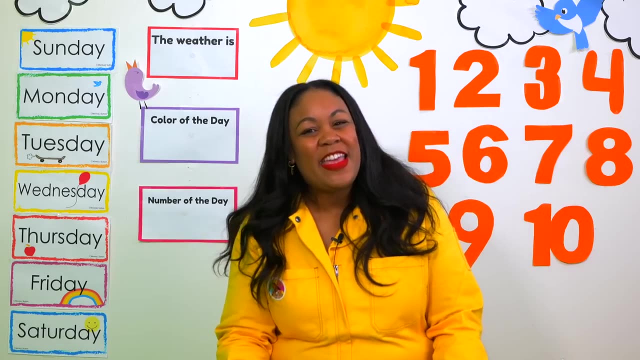 that feelings are what I have. I have many feelings. Feelings are what I have. I have many feelings. Feelings are what I have. I have many feelings. Please don't make me sad. I have many feelings. Can you make me laugh? 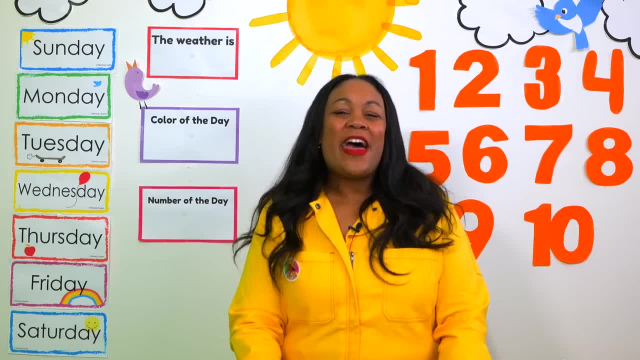 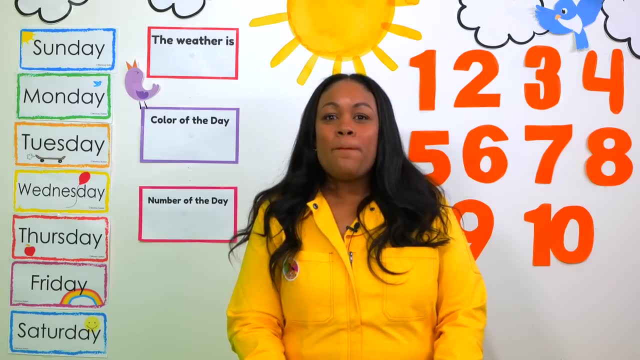 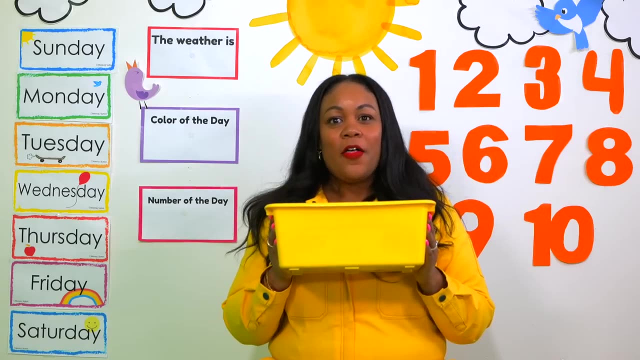 I have many feelings. Feelings are what I have. Oh, we have so many feelings. Thank you for singing with me. Oh, friends, I have a special box I would like to show you. This is my special yellow box. This is my special yellow box. 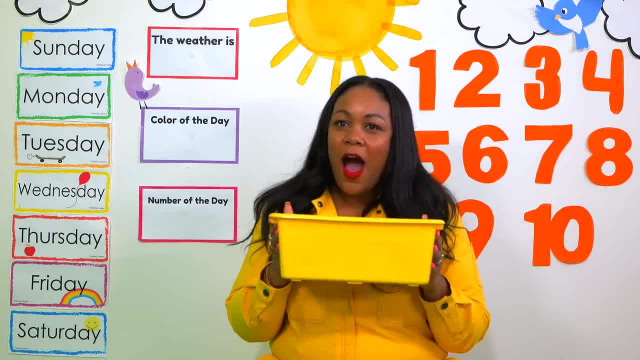 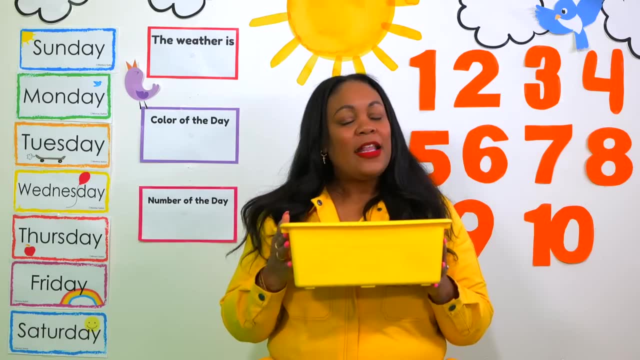 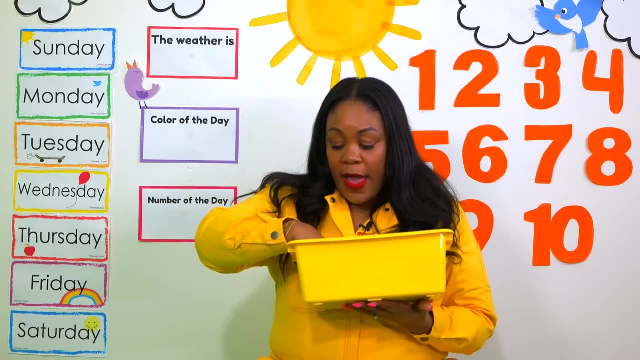 There's so many things inside. Listen, Listen, There's lots of goodies. There's lots of goodies in my box. Let's see what I can find first. Oh, Look at what I found. Oh, let me put it down. I found: 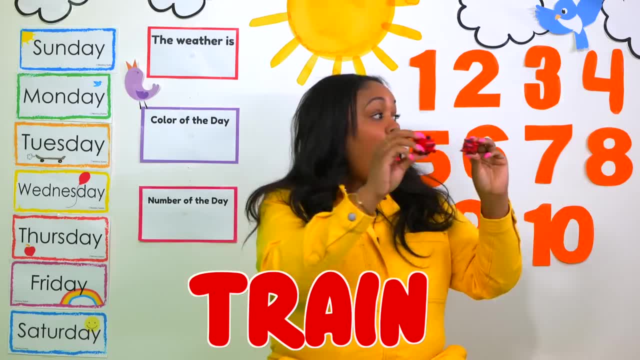 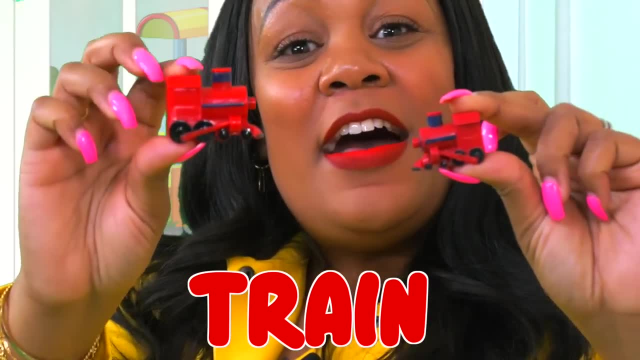 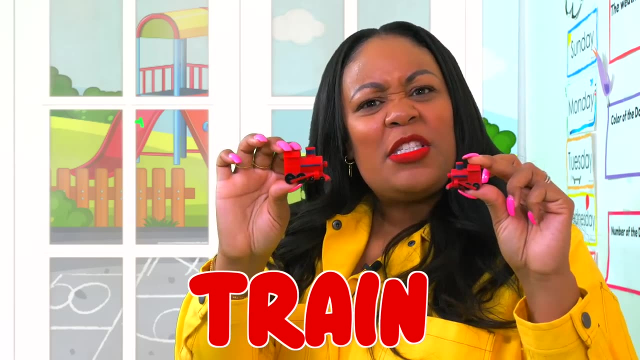 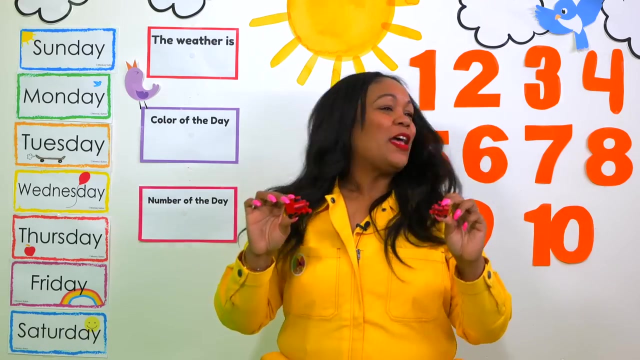 two trains, Two trains. Look at my trains. Wow, Can you say, train Again, Train. These are my toy trains. What sound does the train make? Choo Choo. Can you make that sound? Choo Choo. 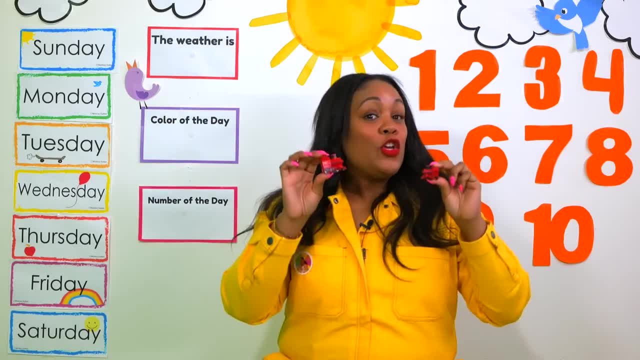 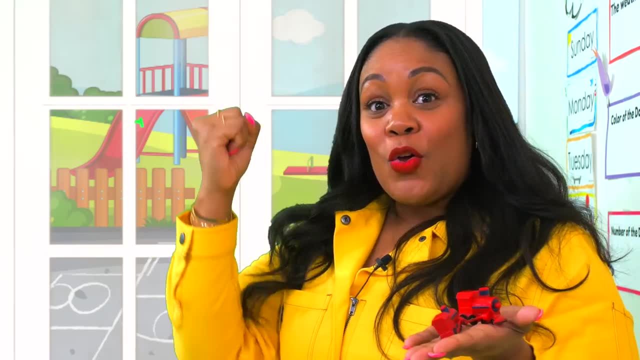 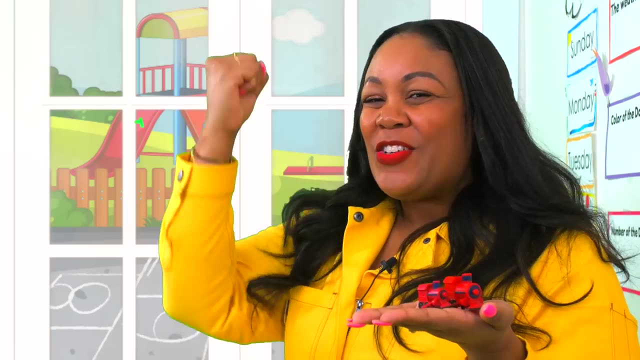 Oh, Let's try it again. Choo Choo. Friends, can you make that sound and go like this? Choo Choo, Let's try it again. Oh, Let me put my train back. Choo Choo. 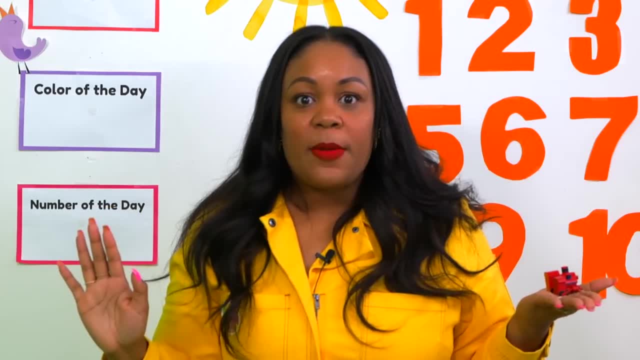 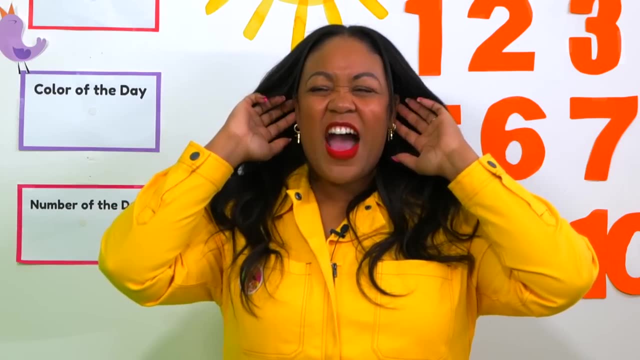 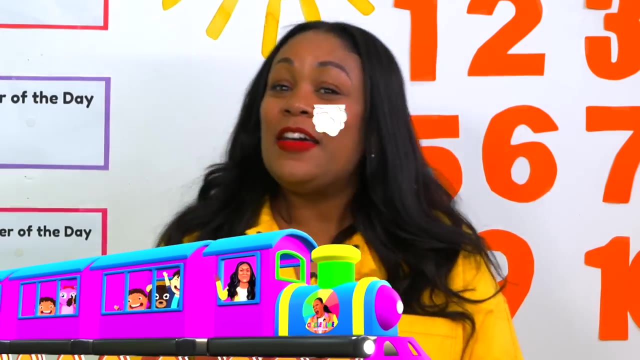 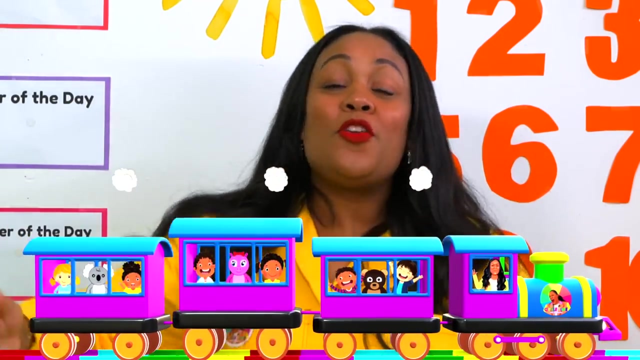 One more time: Choo Choo. Did you hear that? I think I hear something. Listen, Listen, Put on your listening ears. I think I hear our train. The good morning train is coming. How are you? Choo Choo. 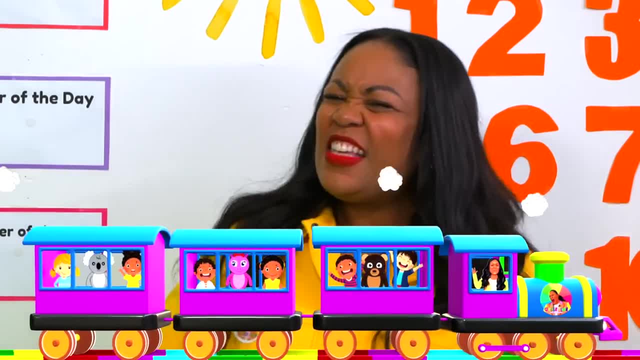 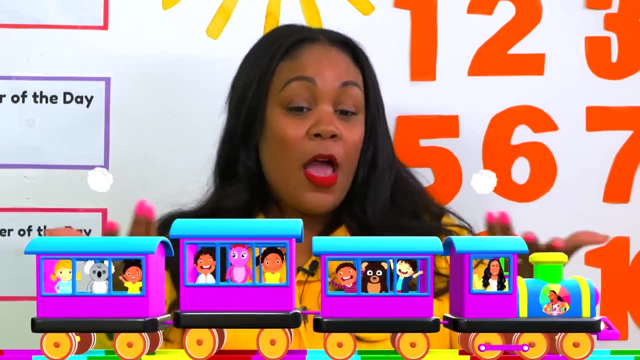 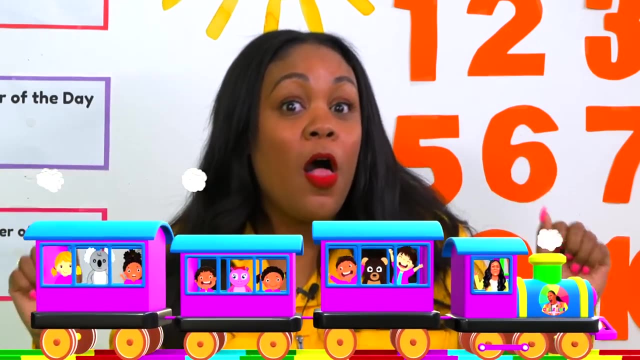 The good morning train is coming. The good morning train is coming. The good morning train is coming. How are you, Choo Choo? And we'll say hello Choo choo. hello friends, And we'll say hello to our friends. 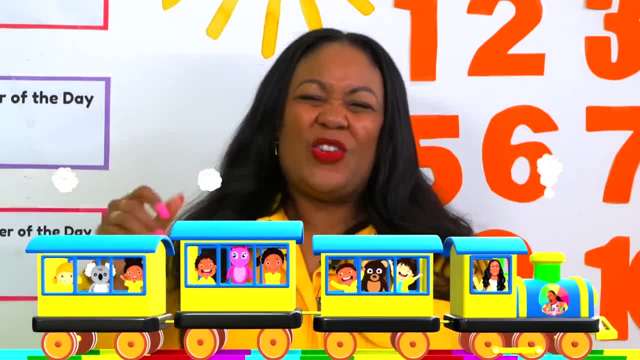 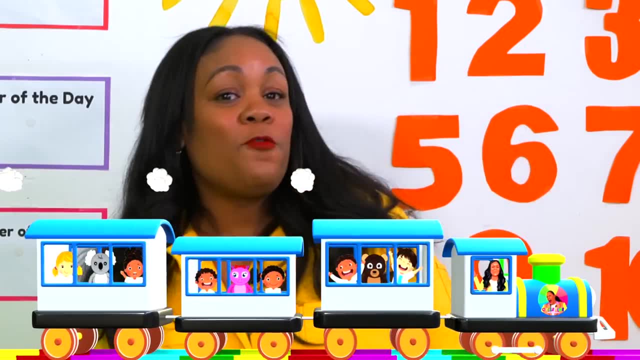 All of our friends wearing Yellow: Choo choo, hello friends. And we'll say hello to our friends. Wearing white: Hello, And we'll say hello to our friends. Wearing blue: Choo choo, hello friends. And we'll say hello to our friends. 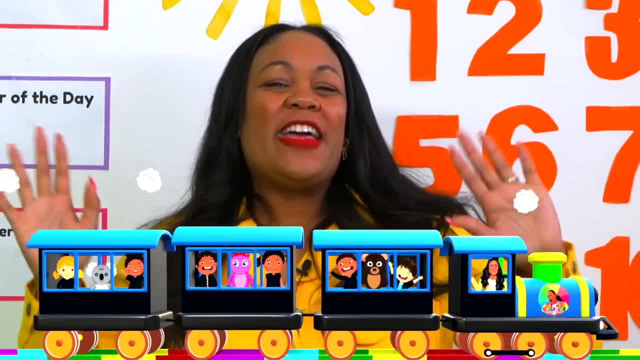 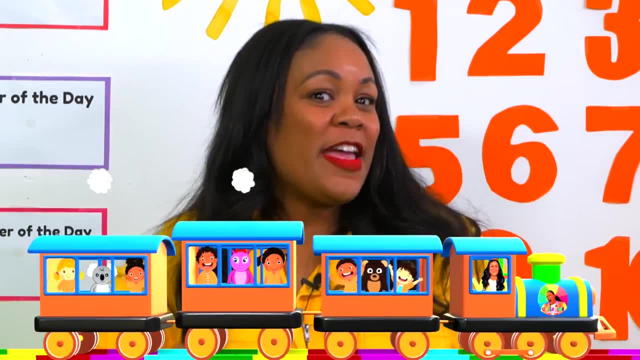 Wearing black: Choo choo- hello friends. And we'll say hello to our friends, All of our friends wearing Orange: Choo choo, hello friends. And we'll say hello to our friends. Wearing pink: Hello, And we'll say hello to our friends. 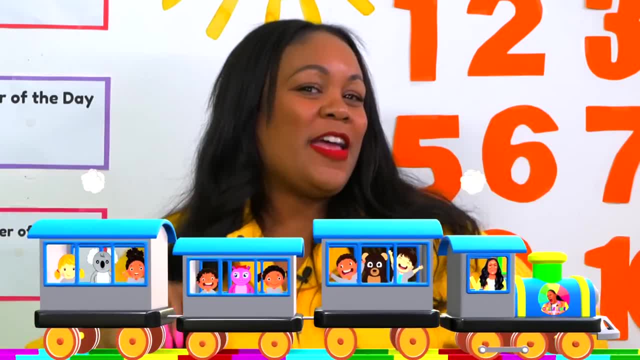 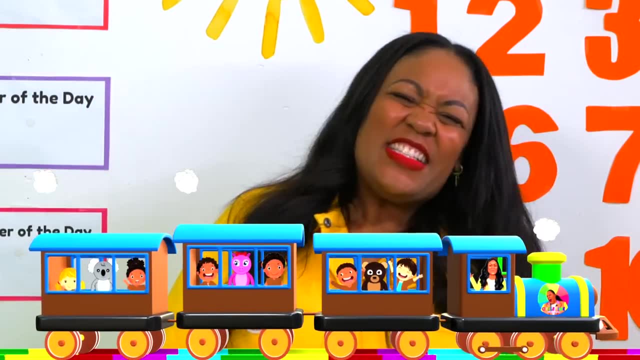 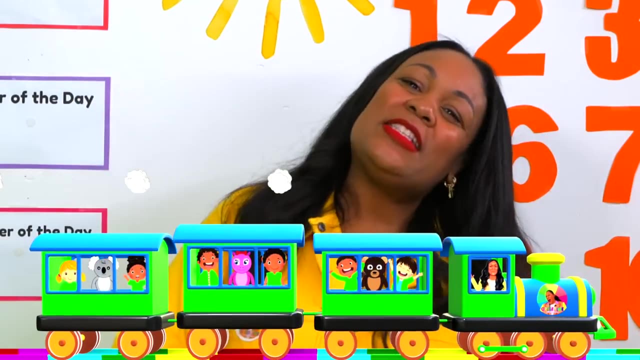 Wearing grey Choo choo: hello friends, And we'll say hello to our friends. Wearing brown Choo choo: hello friends, And we'll say hello to our friends, All of our friends. wearing Green Choo choo: hello friends, And we'll say hello to. 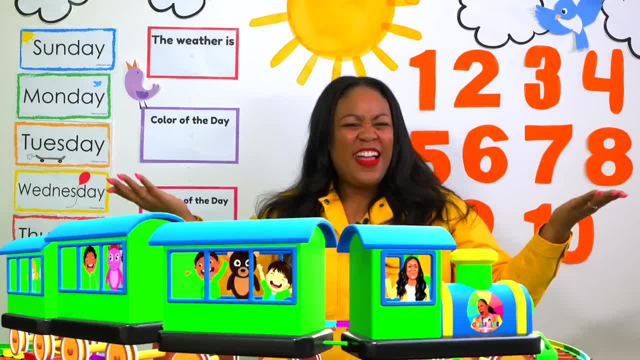 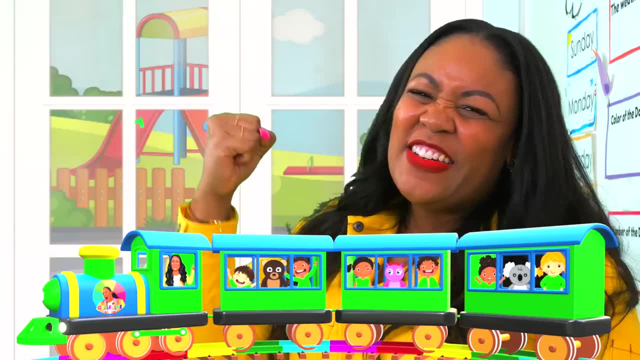 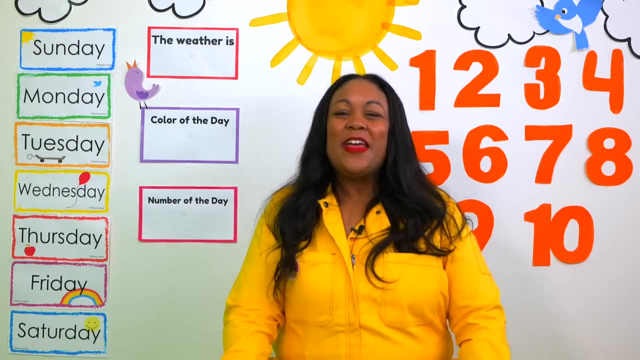 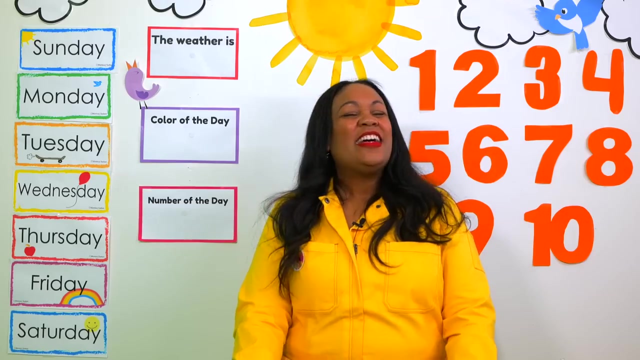 Everyone that's come to Circle. Choo choo. hello friends, Hello friends, Hello friends. Choo choo, Oh, that's my favorite song. Do you like singing that song? Me too. Let's choo choo one more time. Choo choo, Great singing. 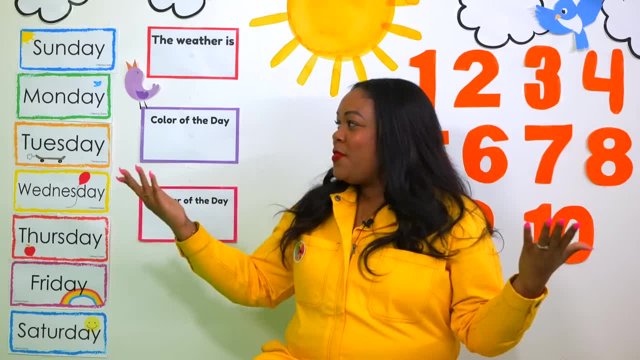 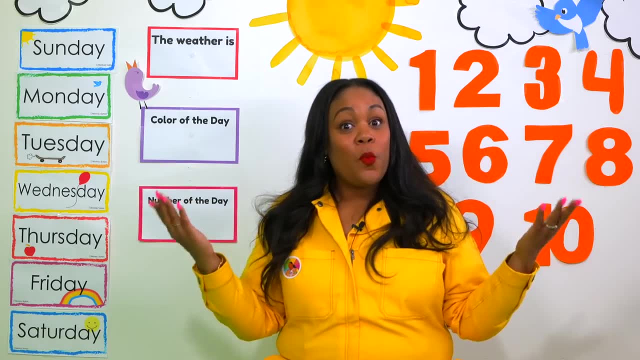 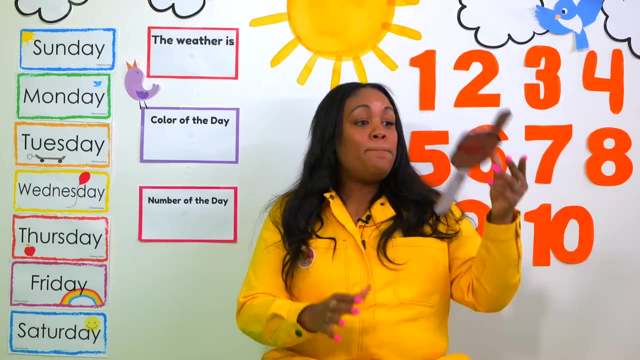 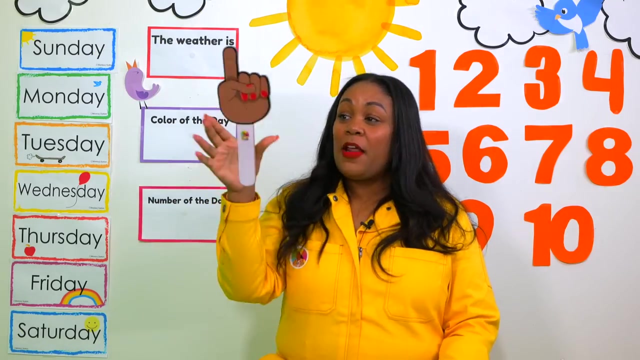 Oh, I would love to show you Some things on our very special board. Oh, how about the days of the week? Oh, but first I need to find my special, My pointer, My circle time pointer, And you can take out a pointer too. Let's look at the days. 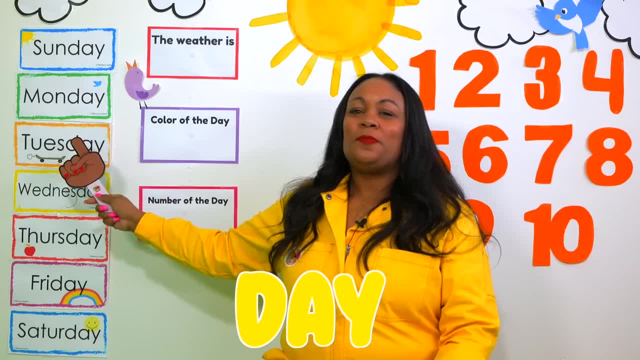 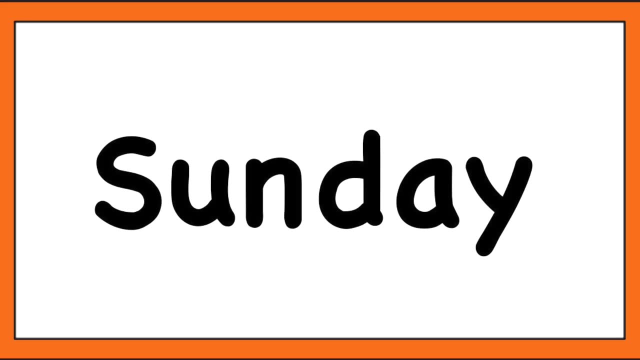 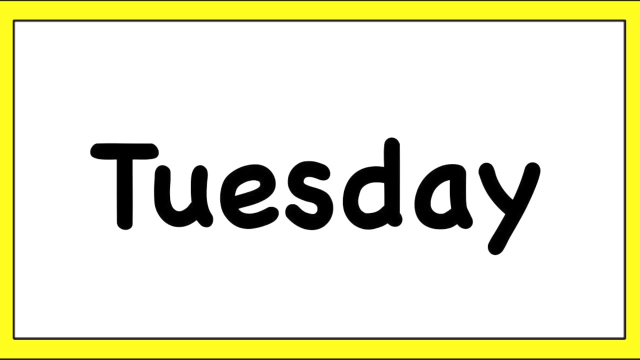 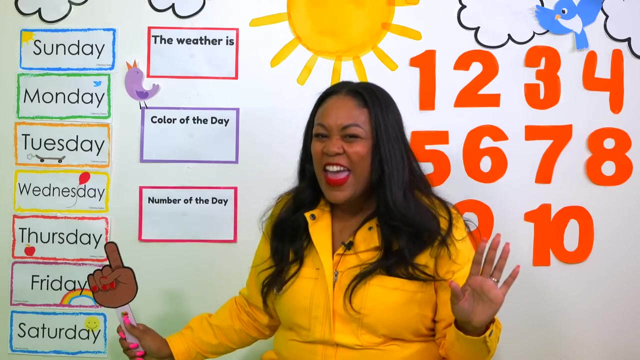 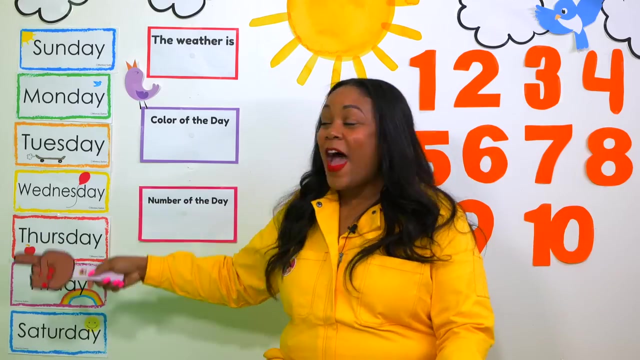 The days of the week. You say day Yes, these are days. There's Sunday And there's Monday, There's Tuesday And there's Wednesday, There's Thursday And there's Friday, There's Saturday And those are our days. I think I'd like to sing a days of the week song. 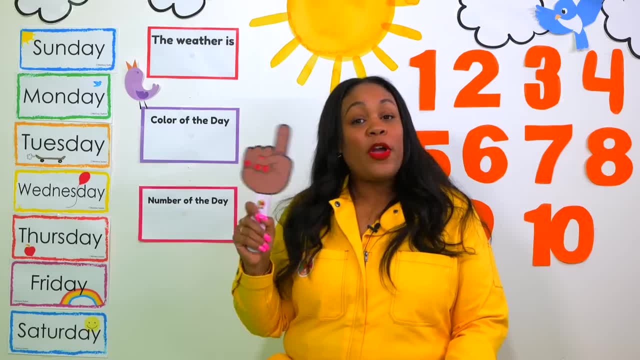 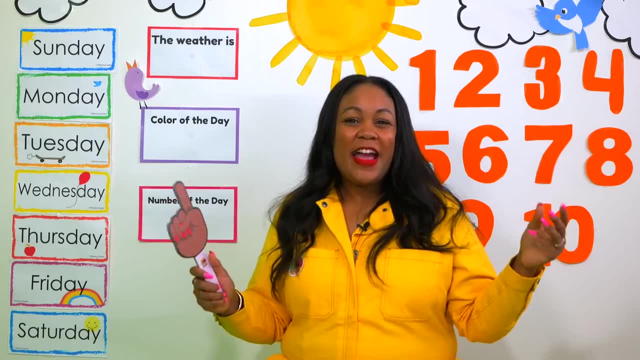 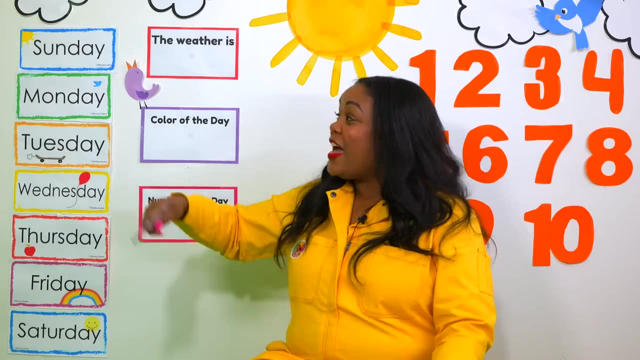 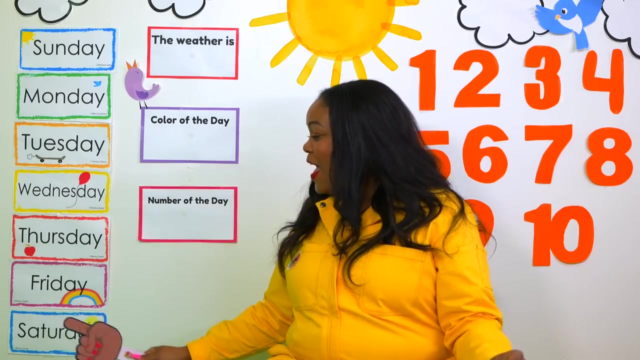 Will you sing with me? Okay, let's point to the days and sing. Here we go, Get ready, Get ready. Here we go. There's Sunday and there's Monday, There's Tuesday and there's Wednesday, There's Thursday and there's Friday, And then there's Saturday. 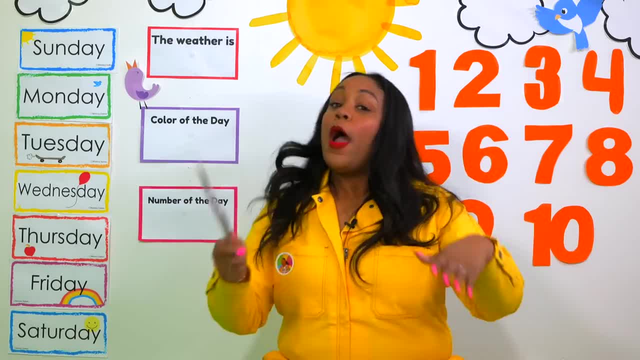 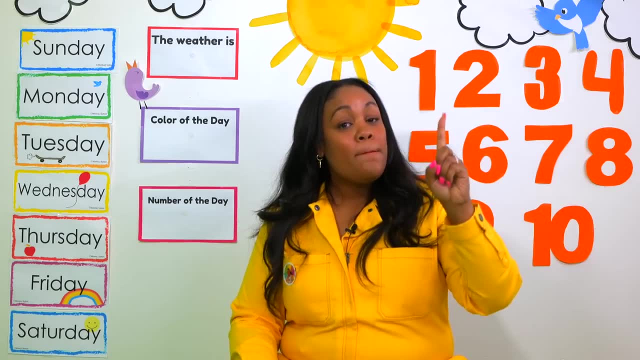 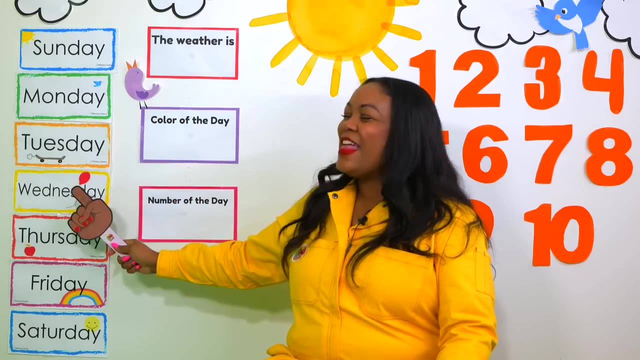 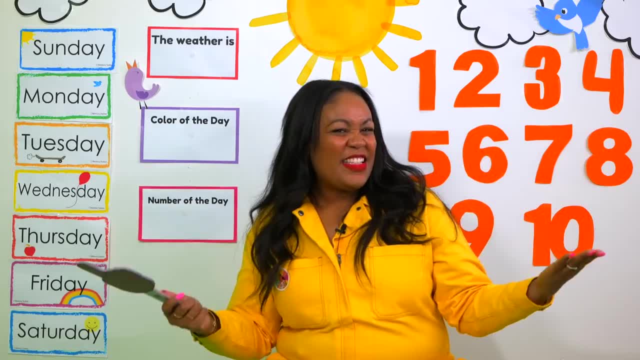 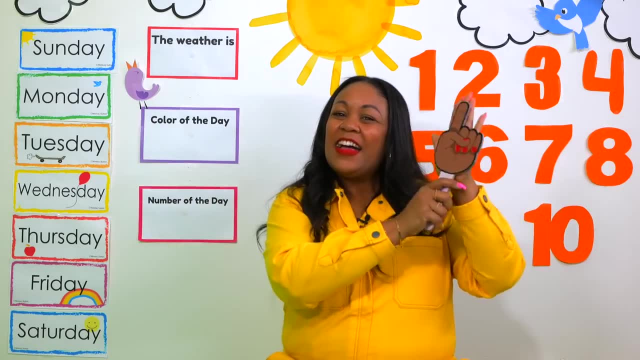 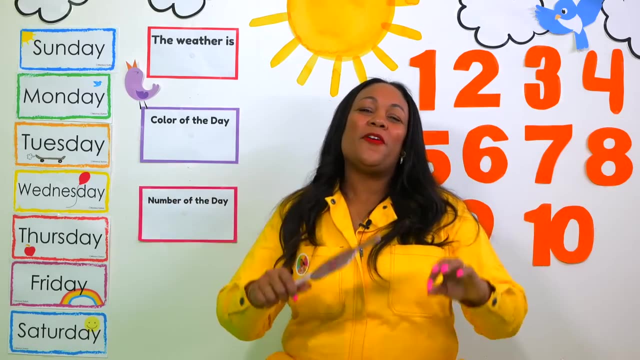 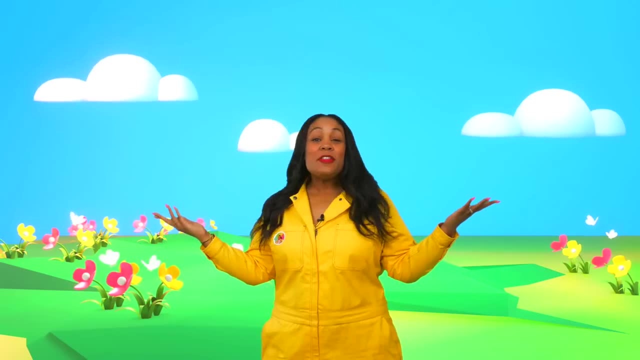 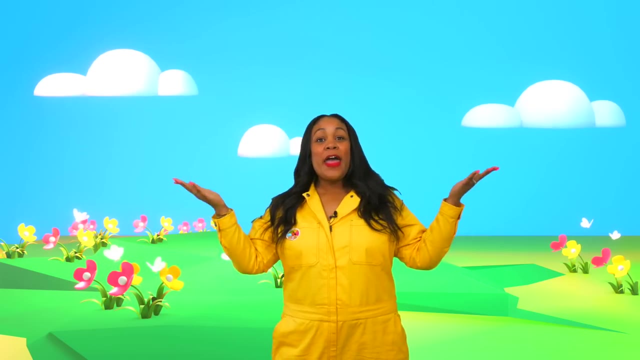 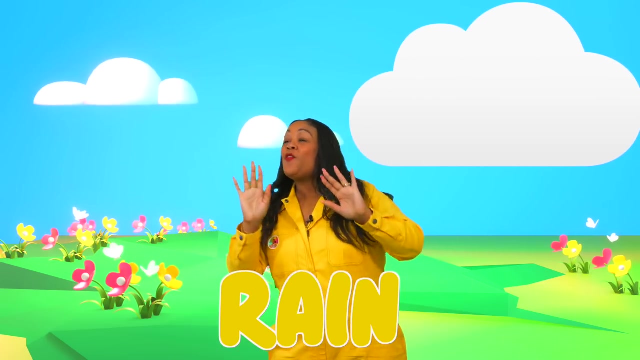 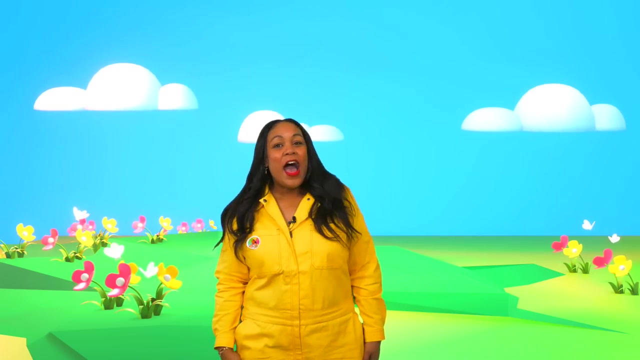 Let's go outside. Come on, We're outside. What's the weather? What's the weather? What's the weather out today? Is it sunny, Is it cloudy, Is it raining out today? Oh friends, What do you see? I see the sun. 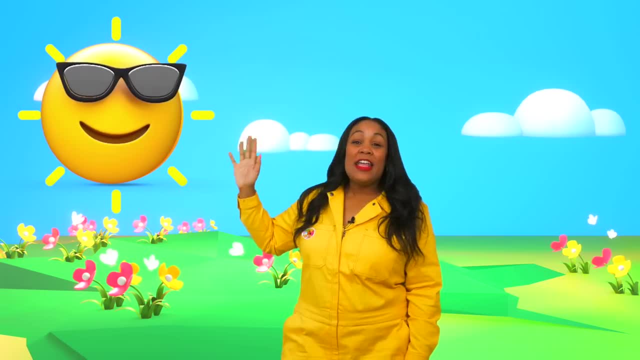 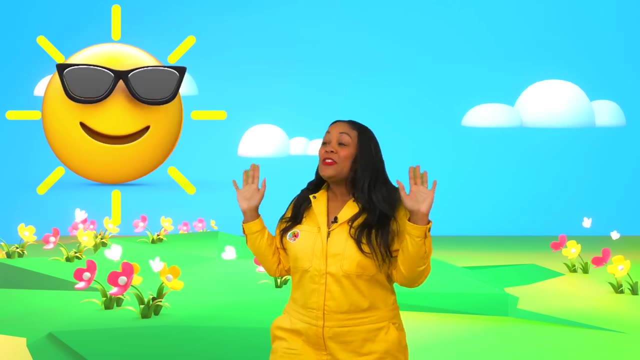 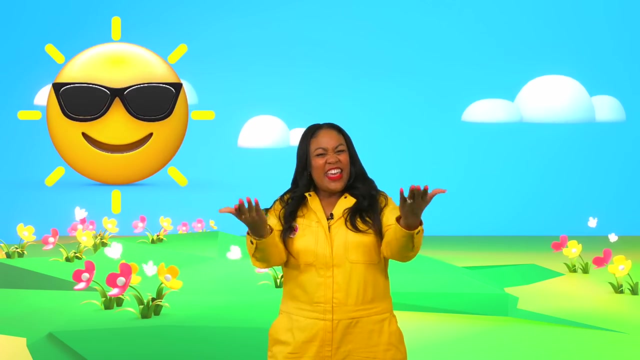 It's a sunny day. Oh, Mr Sun Sun, Mr Golden Sun, Please shine down on me. Oh, Mr Sun Sun, Mr Golden Sun, Hiding behind the trees, These little children are axing you. Oh, won't you please come out So they can play with you. 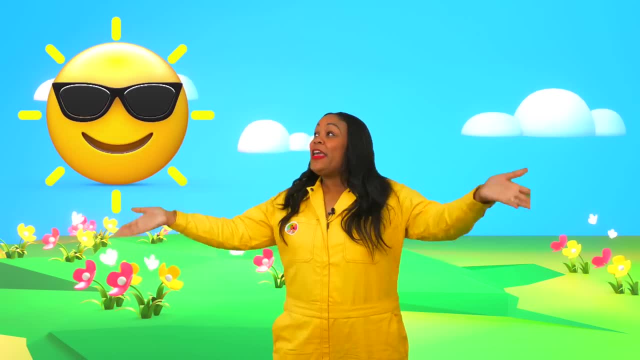 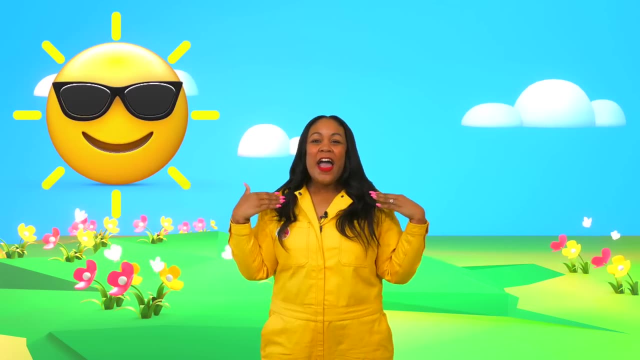 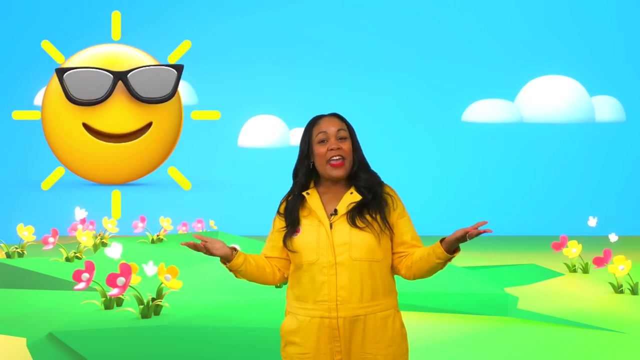 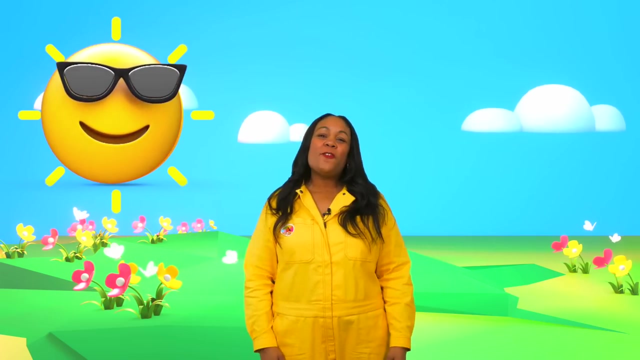 Oh, Mr Sun Sun, Mr Golden Sun, Please shine down on, Please shine down on, Please shine down on me. It's a sunny day. It's a sunny day. Can you say? sunny? Yes, again sunny. It's a sunny day. Now let's help one of our friends get ready for the sunny day. 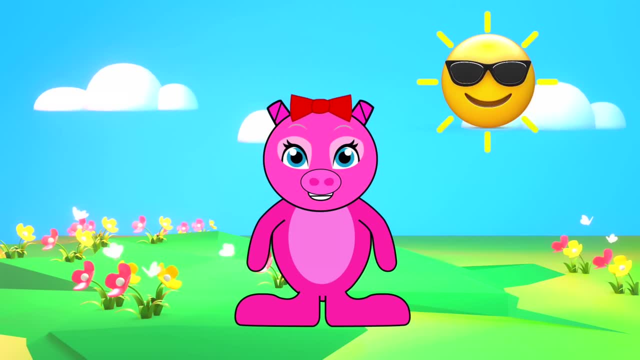 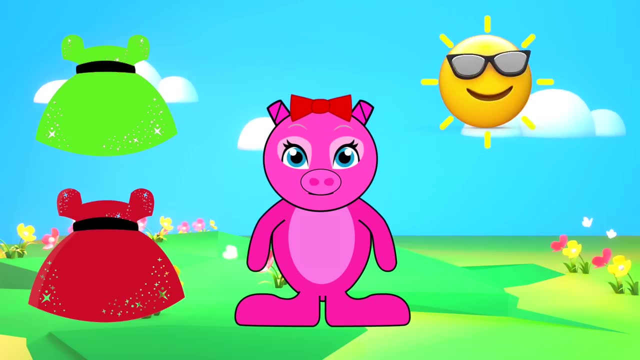 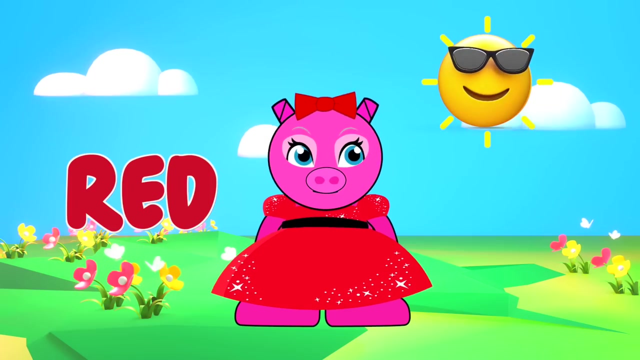 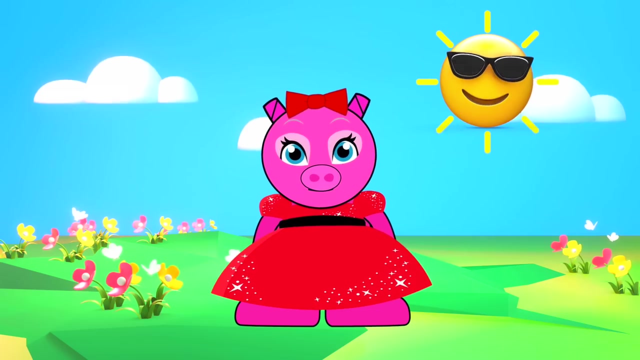 Here we go. Hi friends, Today I would like to wear my red dress. Can you point to the red dress? Point to the red dress? Great Red dress, red dress, red, red red. It's a sunny day out. today I would like to wear my blue sunglasses. 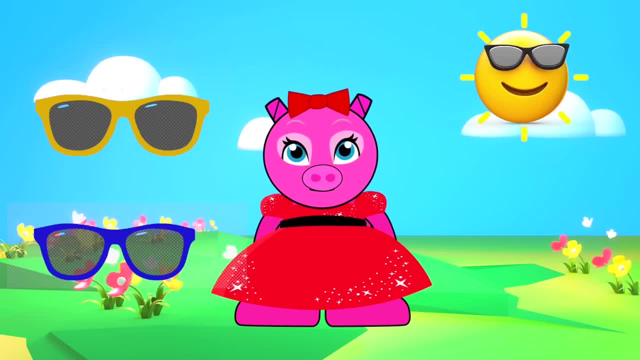 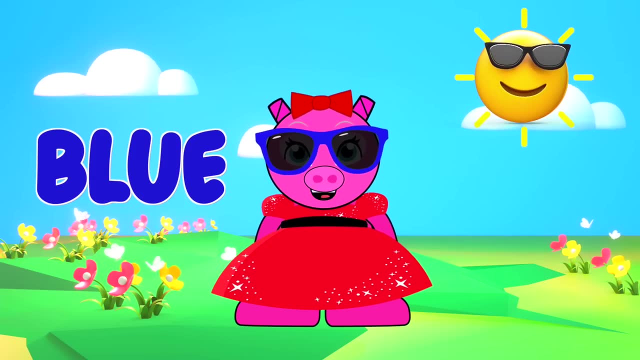 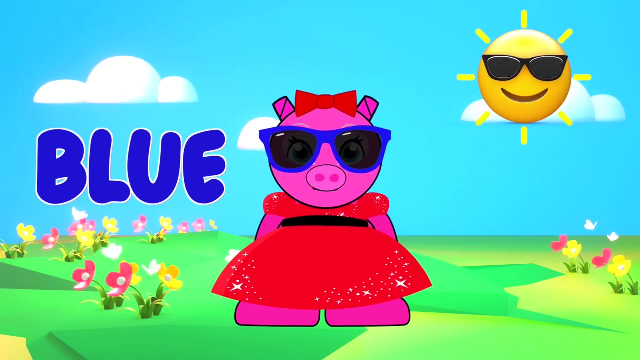 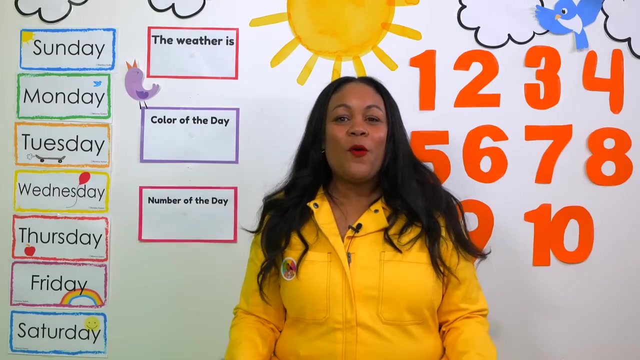 Can you point to the blue sunglasses? Point to the blue sunglasses: Great Blue sunglasses, blue sunglasses, Blue sunglasses, blue blue blue. You did it, Thank you, friends. Bye, Oh, I'm so happy we went outside together. Oh, friends, 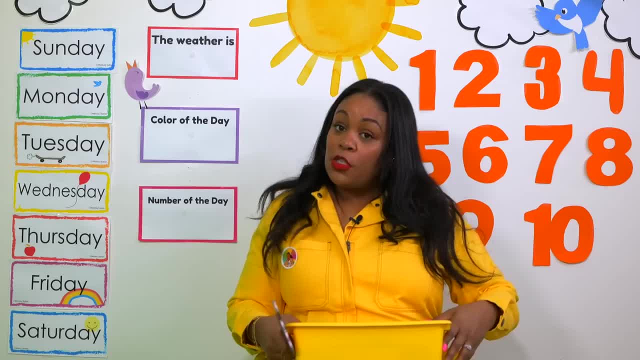 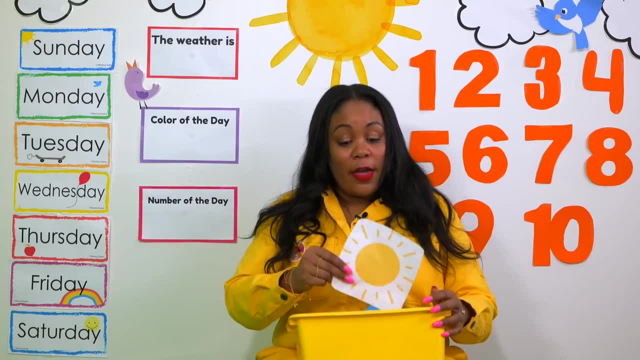 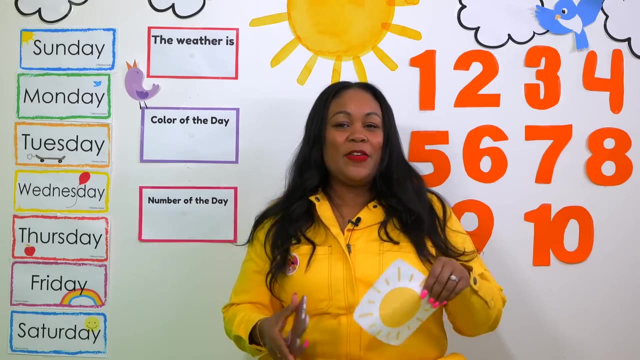 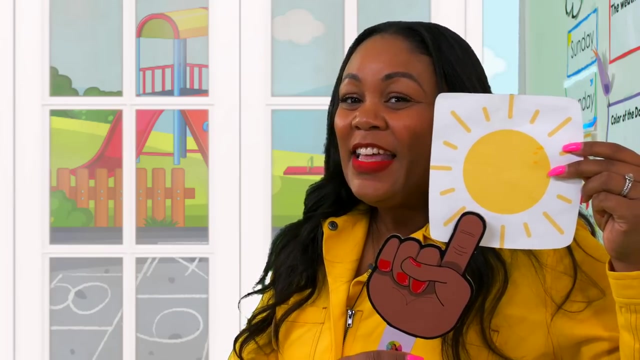 I wonder if I have a sunny day picture to put on our board. Let me look. Oh, look at this. I think I do have a sunny day picture. Oh, can you say sunny? Yes, Can you say sunny? This is a picture of a sun. 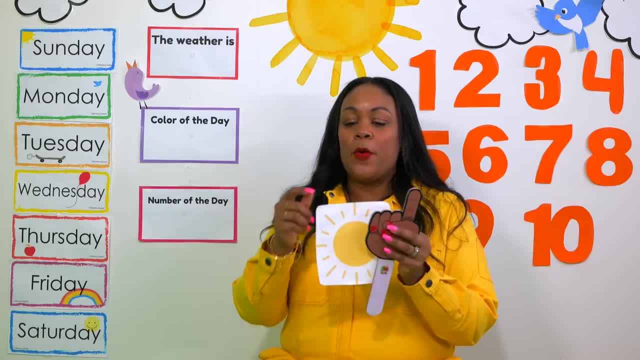 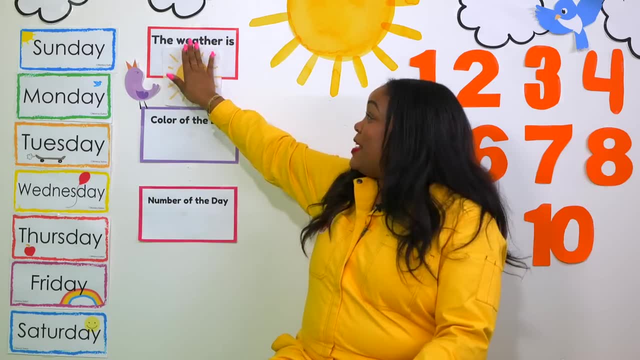 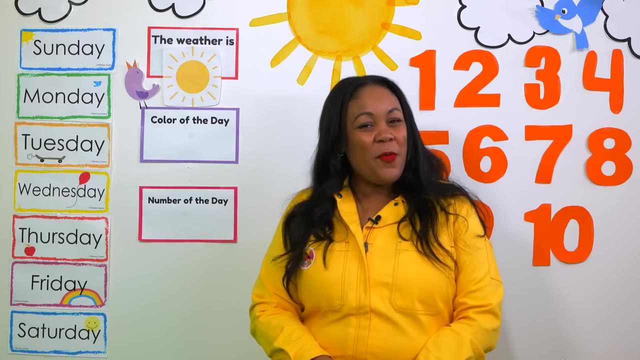 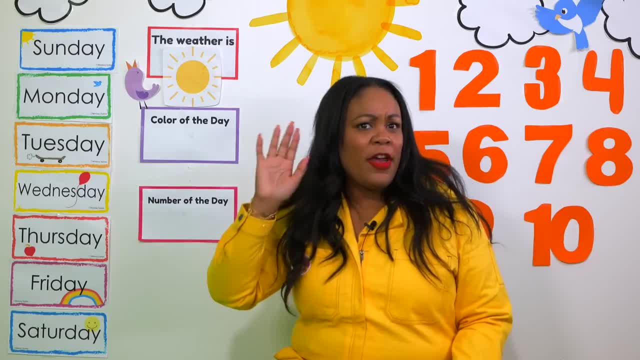 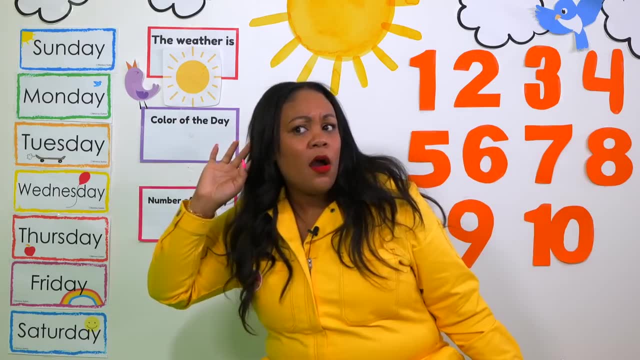 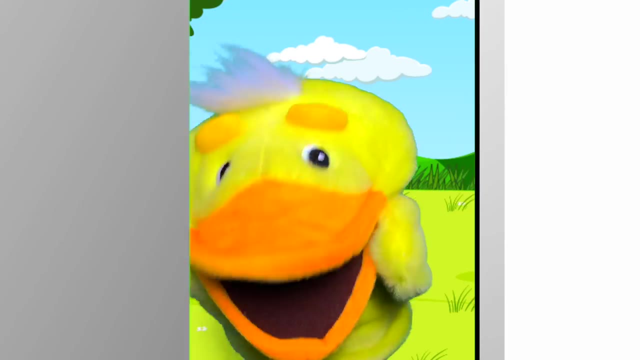 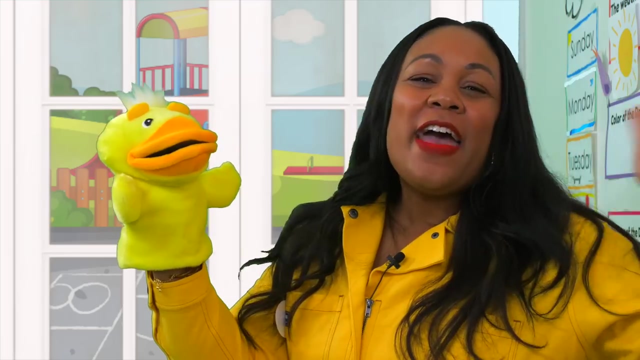 Oh, did you hear that? I think I hear a doorbell. Listen, everyone, Listen, Listen with your ears, Listen Who is it? It's Tuk Tuk. Hello, Tuk Tuk, Hello friends. Oh, everyone wave to Tuk Tuk. 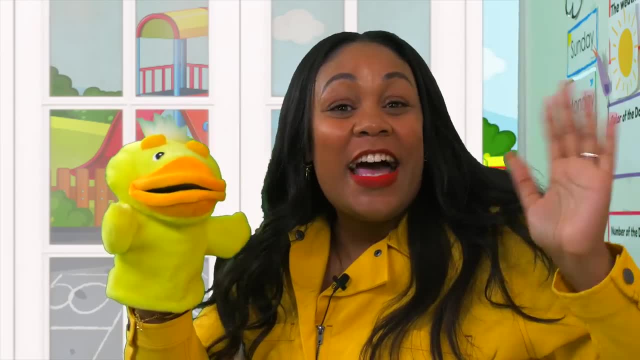 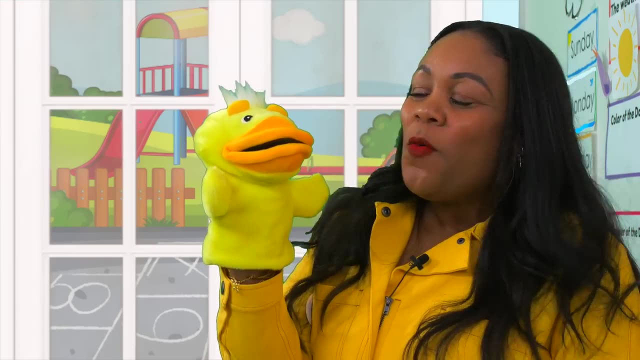 Hello Tuk Tuk, Hello Tuk Tuk, Hello Tuk Tuk, We're happy you're here today. Hello Tuk Tuk, We're so happy you're here today. I'm happy to be here, friends. 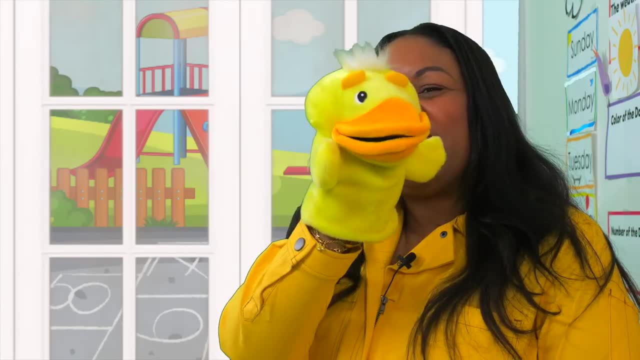 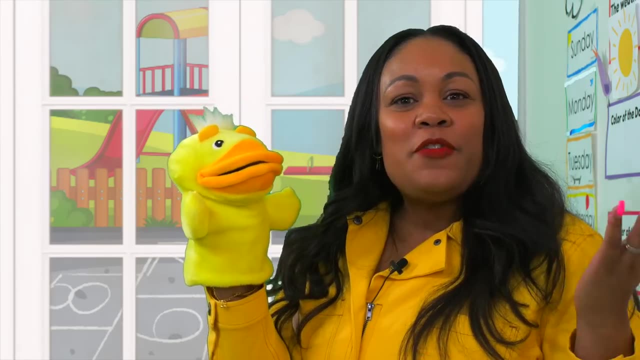 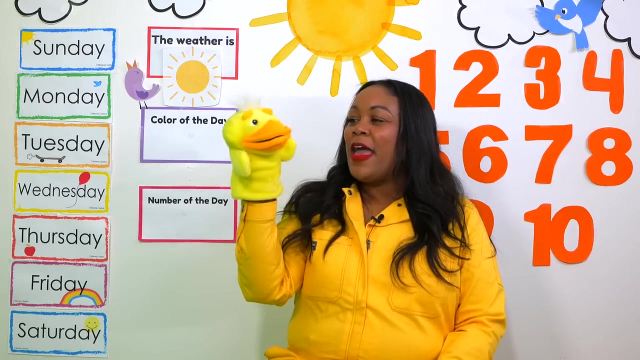 How do you feel today? Tuk Tuk, I feel good. Oh Tuk Tuk feels good. Oh Tuk Tuk, we have so much to do. Let me show you our new classroom. Look, Wow, It's beautiful, Miss Monica. 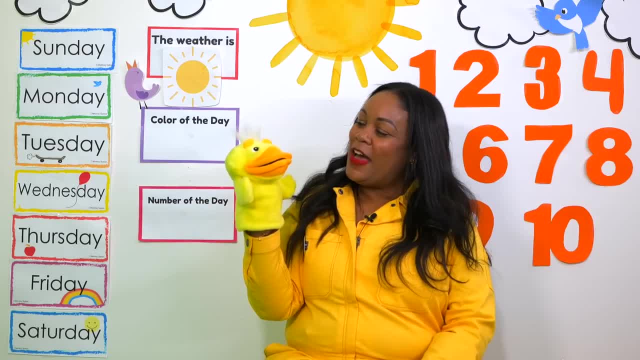 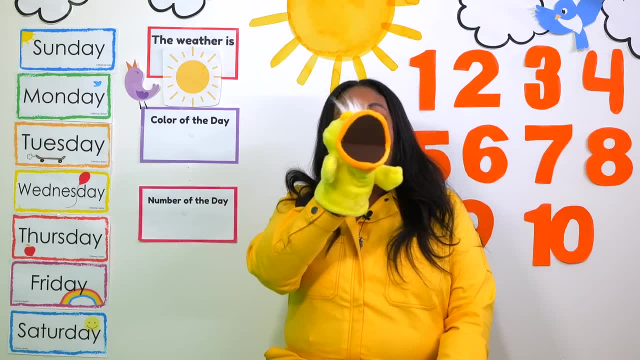 Oh, I'm so happy you like it. Tuk Tuk, Oh, Tuk Tuk. guess what Today, I think we're going to get a special delivery, Really, Yes, Oh friends, Did you hear that? 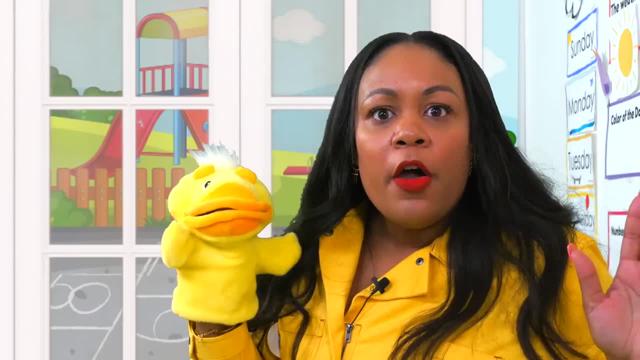 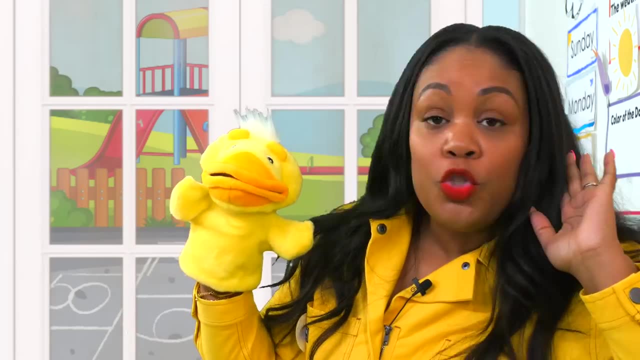 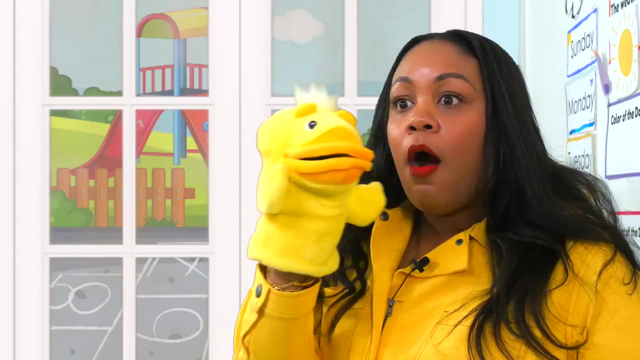 I think I hear a horn Horn. Did you hear a horn? Listen, Tuk Tuk, listen, Friends, listen. Do you hear a horn? Ooh, Tuk Tuk. do you hear the horn? I do. 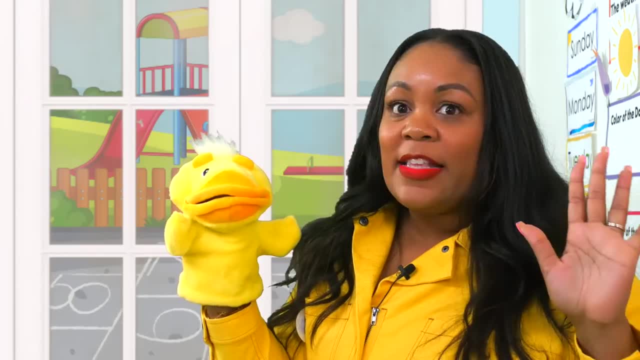 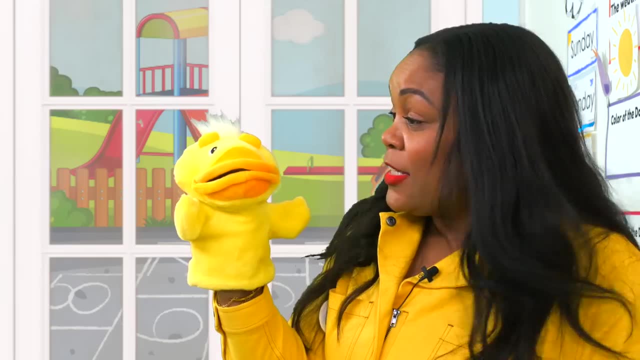 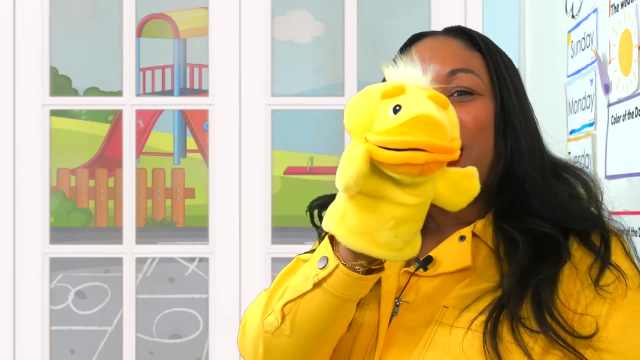 Maybe it's the delivery person. Let's listen again. Package for Miss Monica. It is. We have a special delivery. Tuk Tuk, will you go outside with me to the mailbox? Yes, Miss Monica, Let's go friends. 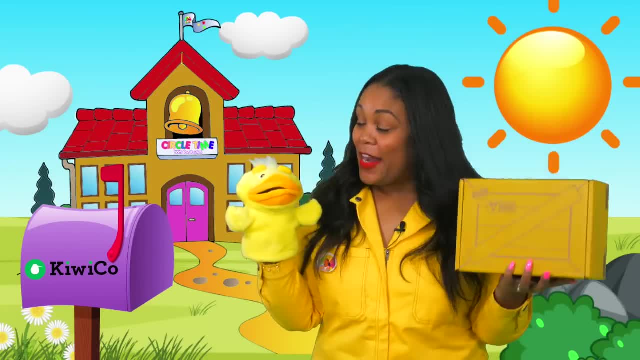 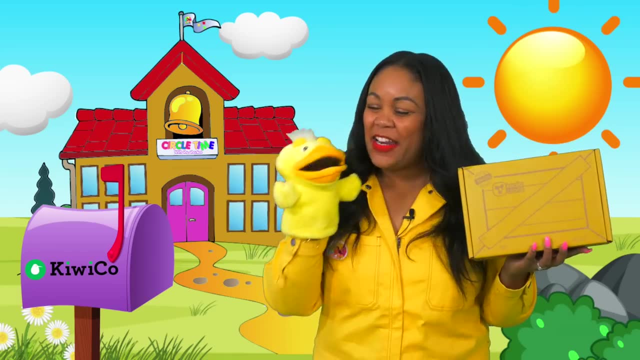 Here we go, Tuk Tuk. look at what we got in the mail today. It's our koala crate from KiwiCo. I can't wait to see what's inside Me too. Oh, I can't wait to see what the surprise is this month. 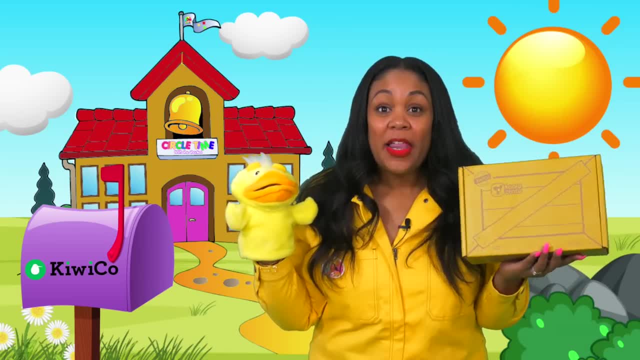 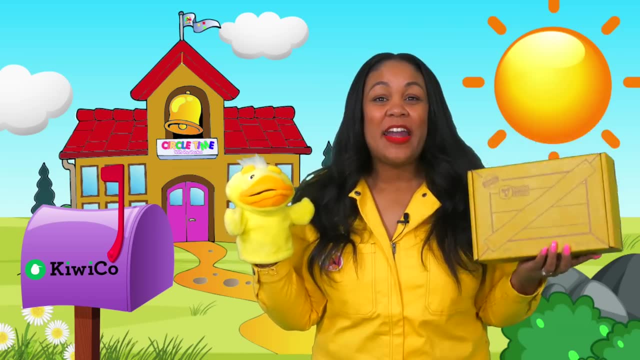 Oh, friends And Tuk Tuk, do you want to go inside so we can play? Yay, Oh, I do too. Okay, let's go inside and we can see what's in our koala crate. Here we go. 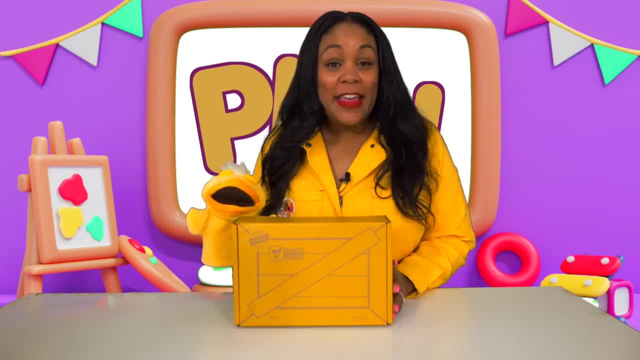 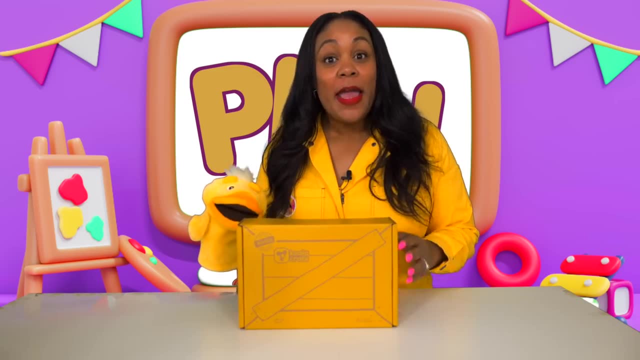 Come on everyone. Oh boy, Tuk Tuk, I can't wait to open up our koala crate. Are you ready? Yes, yes, Okay, friends, let's count to three and we'll open up the koala crate and see what's inside. 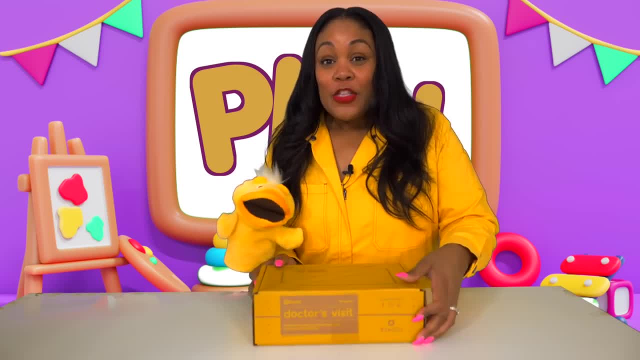 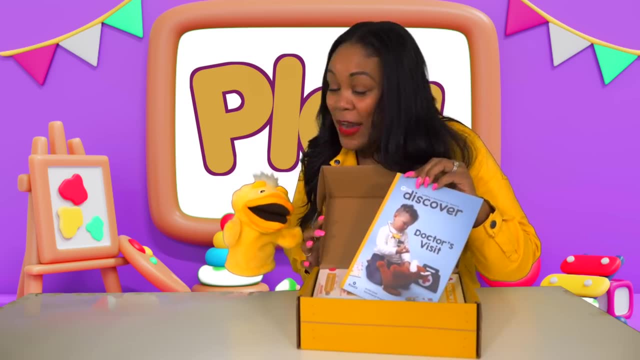 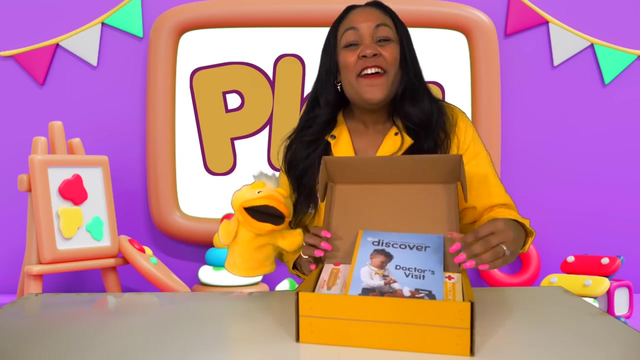 Let's see what the surprise is. One, Two, Three, Wow, We're going on a doctor's visit. Yay, Tuk Tuk, are you excited? Yay, We're going on a doctor's visit. Tuk Tuk, doctors, take care of us. 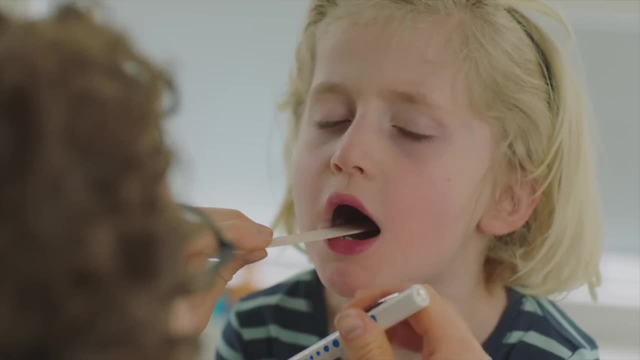 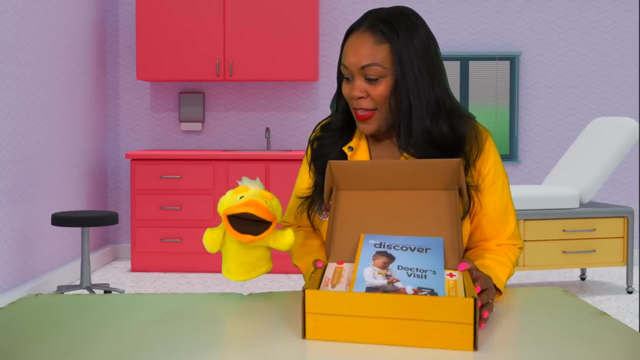 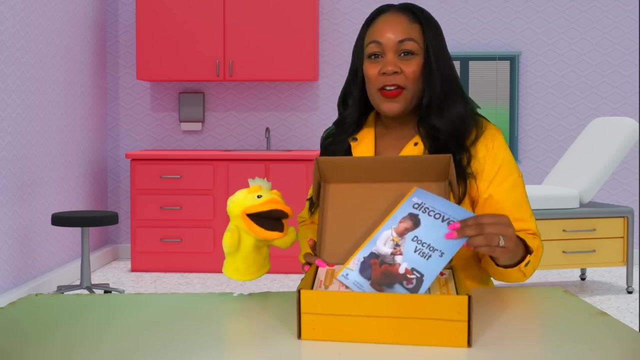 They make sure we're feeling okay. If we feel a little bad or sad, we can go to the doctor and they can help us. Do you want to play doctor today? Yes, yes, All right, Me too. Okay, let's see what's in our koala crate. 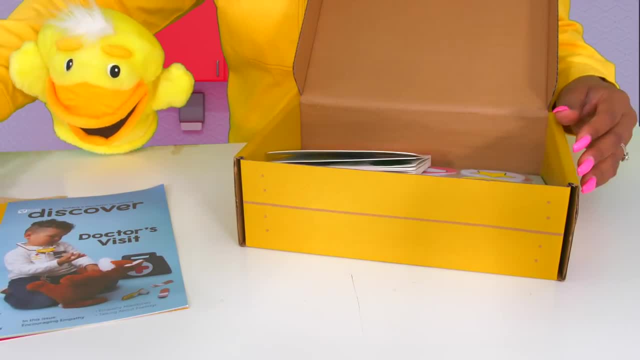 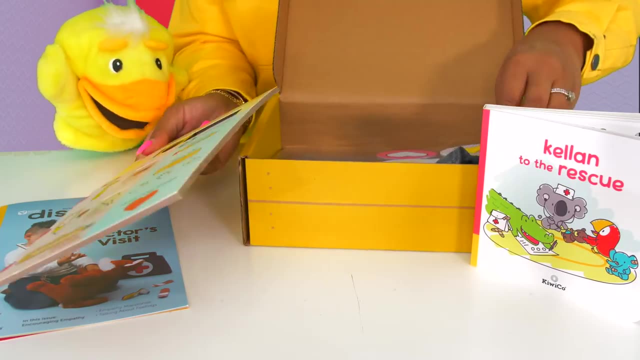 Let's take some of the things out. Wow, There's so many things inside, Everything we need. Tuk Tuk, We can read a book. Kellen to the rescue. There's a doctor's checklist. Oh, you can check the patient. 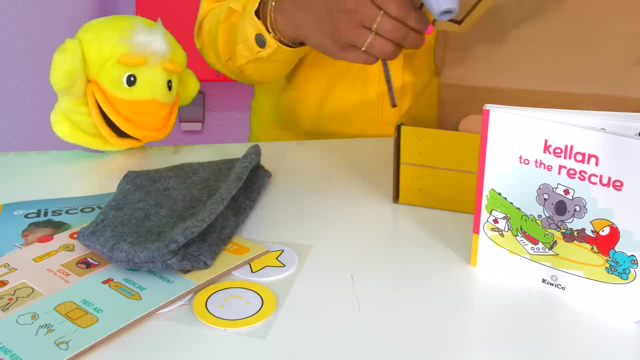 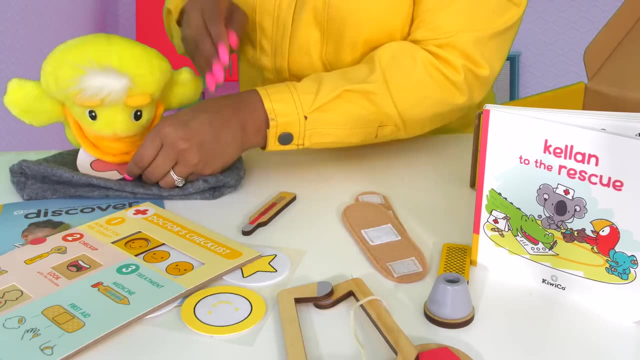 There's stickers, Oh, and a bag that we can use for our medical kit. All right, let's put the medical tools in our bag, Oh, but first put the sticker on Tuk Tuk, Tap, tap, tap. 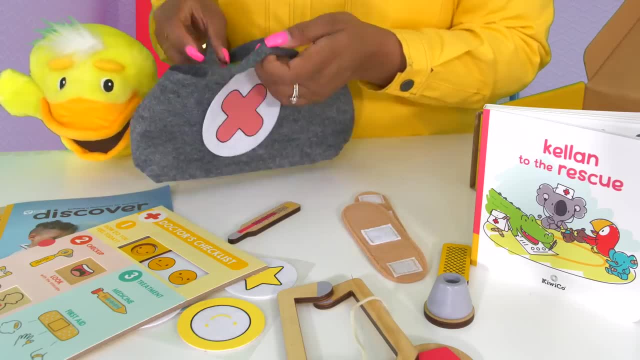 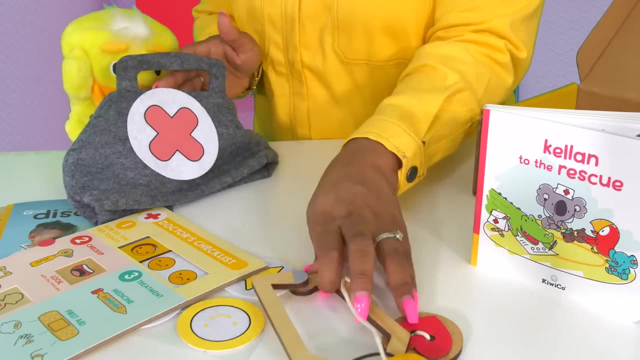 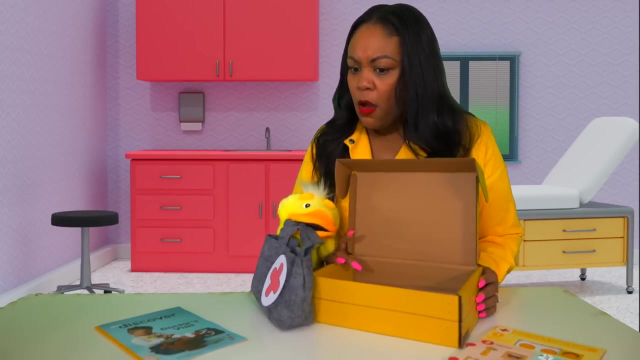 Thank you. Now we can put the medical tools inside. Hold it open: Bandage thermometer. we have an otoscope and a stethoscope. I think we're ready. Let's play. I think we need a patient. Maybe I can get one of my dolls. 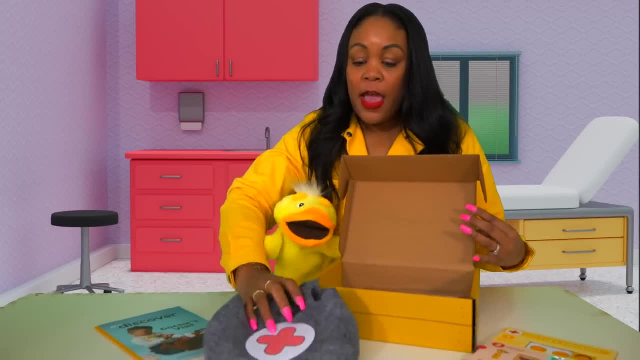 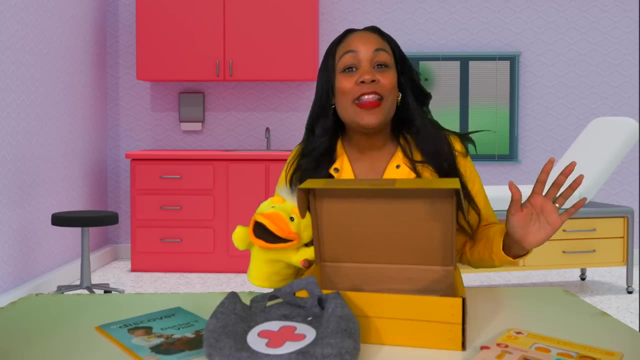 Okay, let's get one of our dolls, Tuk Tuk, and we can play doctor. Are you ready? Quack, quack. Yes, Tuk Tuk's ready. Okay, let me find one. Okay, let me find one of my dolls. 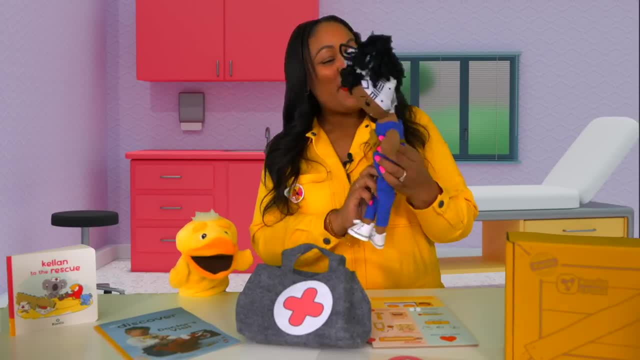 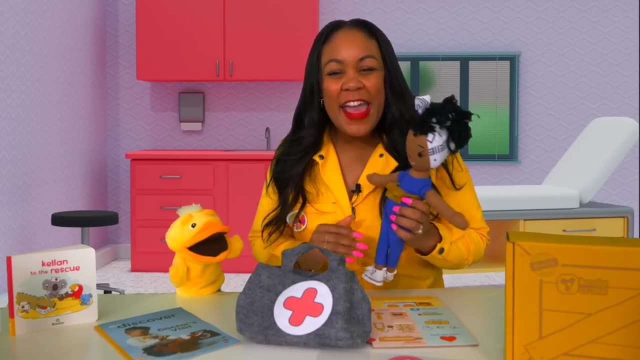 I'll be right back. Yay, Here's my doll, Mia. Mia can be the patient. Mia, do you want to play? Yes, yes, yes, I want to play. All right, Mia's going to be the patient. 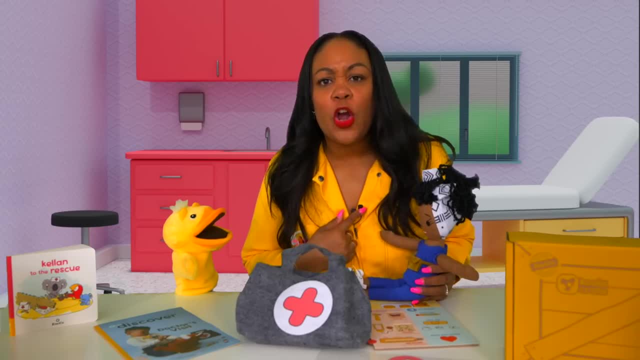 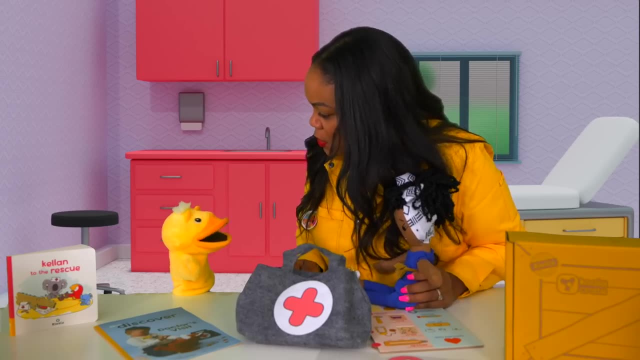 Tuk Tuk, I want to be the doctor. Will you be the doctor's assistant? Oh, better idea. How about, Tuk Tuk, You can be the nurse. Do you want to be the nurse? Quack quack. 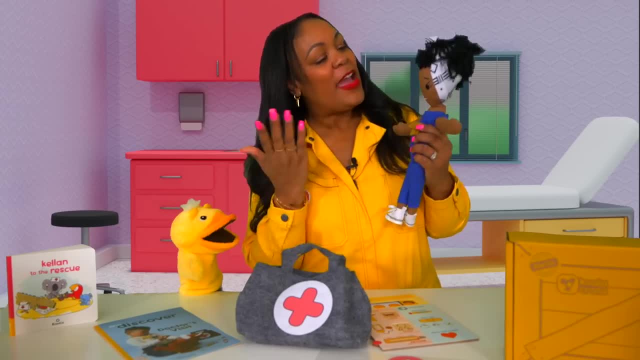 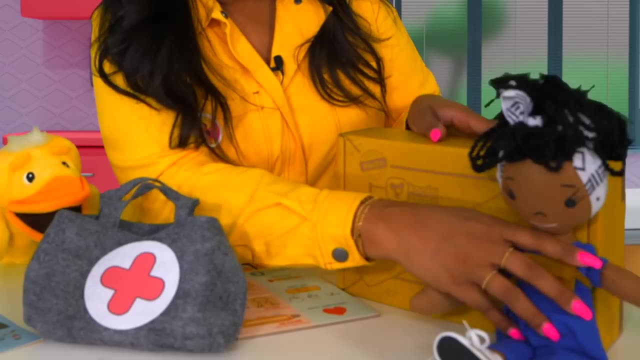 Yes, Tuk Tuk is going to be the nurse, Mia is going to be the patient. Okay, let's find some place for Mia to sit. You can sit right here, Mia, Have a seat. Oh, sit right here. 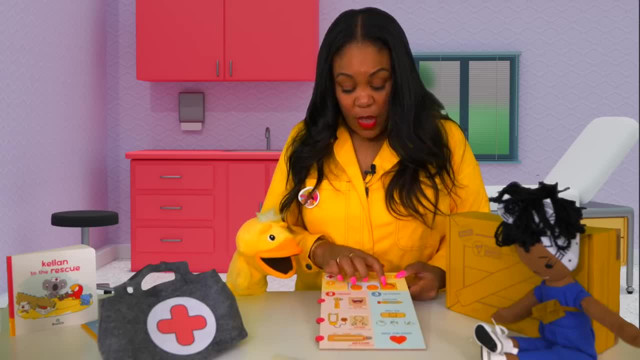 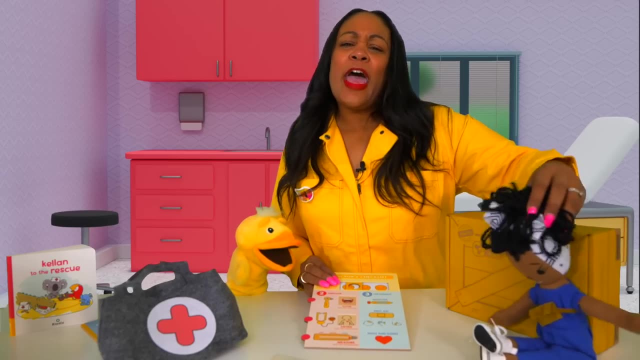 Tuk, tuk, tuk tuk. How do you feel today? Do you feel happy, Do you feel just okay Or sad? I feel sad today. Oh, Mia feels sad. Let's put sad Tuk Tuk. 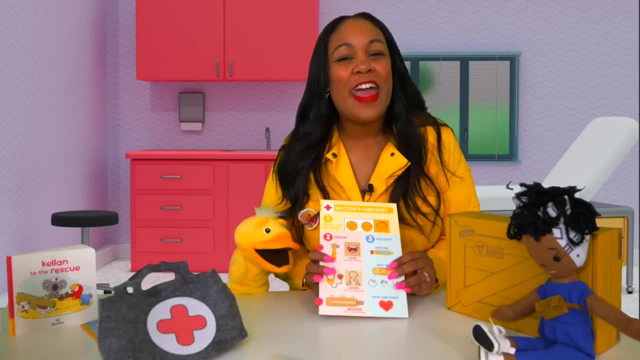 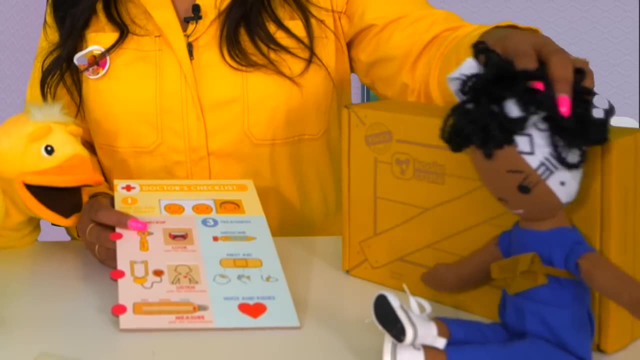 You see, Yes, Quack, quack. Okay, Mia feels sad. Oh Mia, why are you sad today? Oh, my tummy hurts and I fell down too. Oh no, Mia fell down and her tummy hurts. 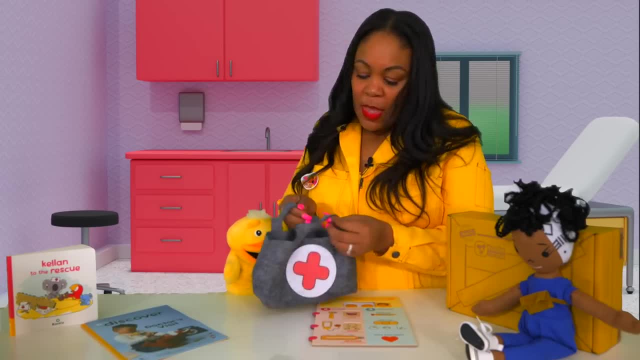 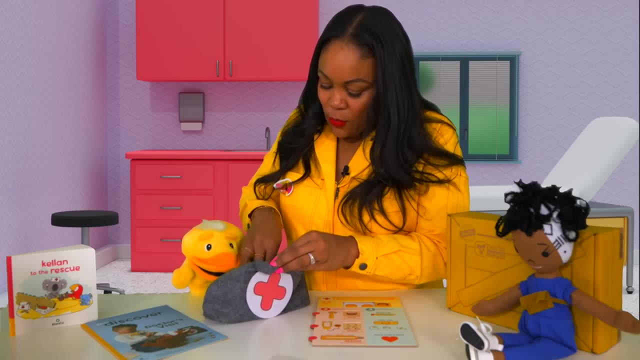 Mia, let's take your temperature. Let's see what's inside the medical doctor's bag. Okay, Tuk Tuk, help me open. Hold it right there. Tuk Tuk, Thank you. Oh look, We have a thermometer. 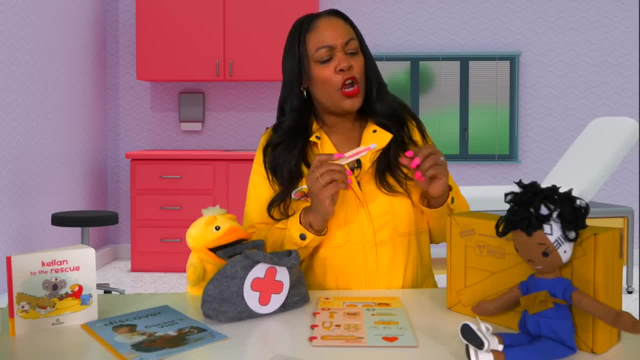 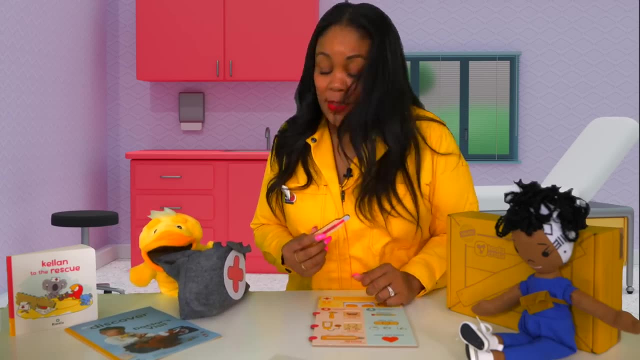 Look, Tuk Tuk, Mia, we can take your temperature. The thermometer will let us know: Is Mia feeling really hot Or is Mia's body really cold? Let's see. Okay, come over here, Mia, Lift up your arm. 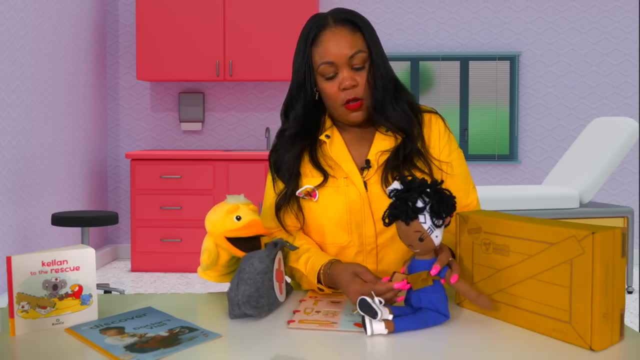 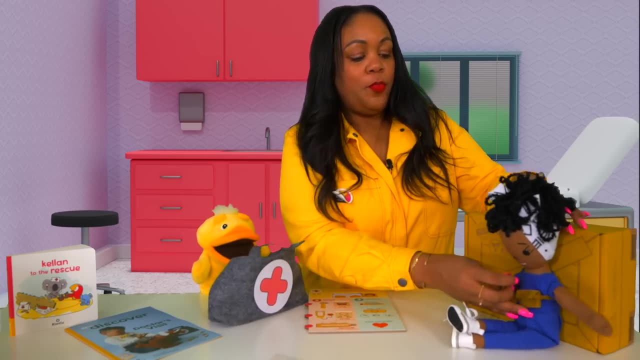 We'll put it right under there. Hmm, Tuk tuk, tuk, tuk, tuk tuk. Oh, I think. Oh, let me see, I'll have to put this on our chart. Mia is feeling warm. 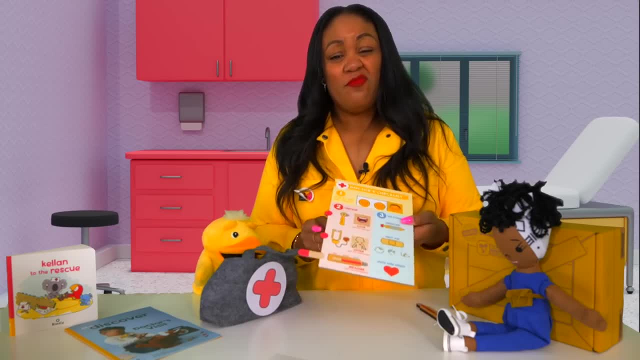 You feel a little warm today, Mia, A little warm, Okay. And you said: you fell down. Yes, I fell down. Oh, where did you hurt yourself, Mia? Oh, on my knee. Oh, let's get Mia a bandage. 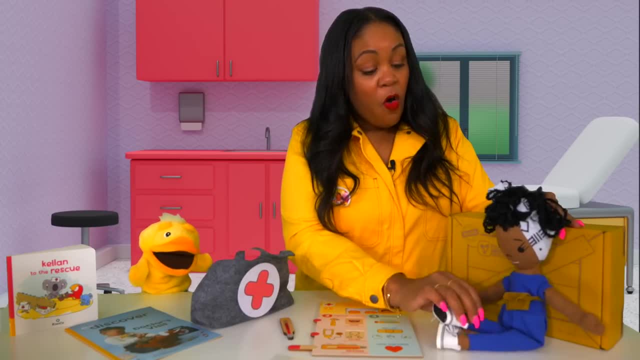 Open the bag. Tuk Tuk, Yep, Okay, I think we have a bandage. Can you hold the bandage? Tuk Tuk? Good job, I'll put the bag here. Thank you, Tuk Tuk. 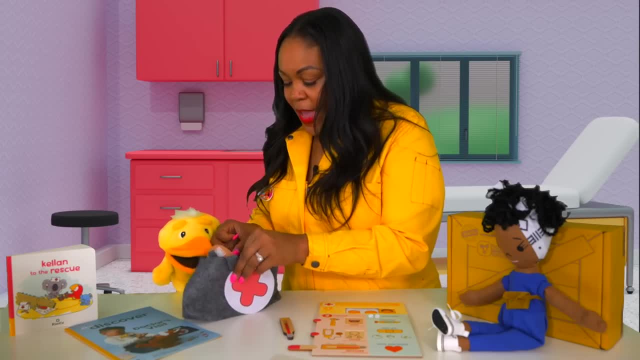 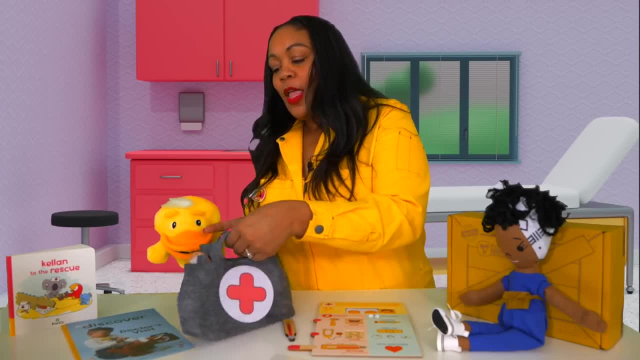 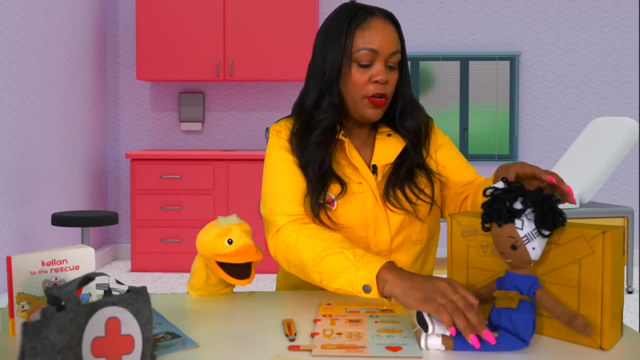 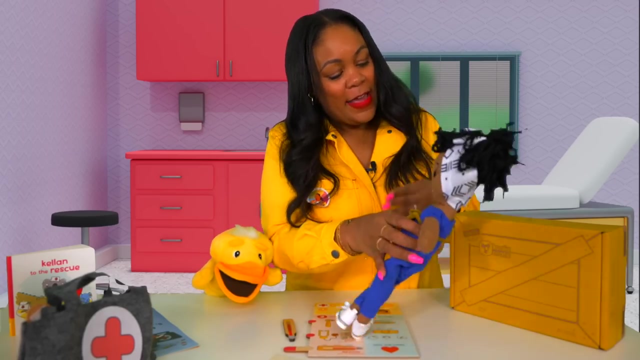 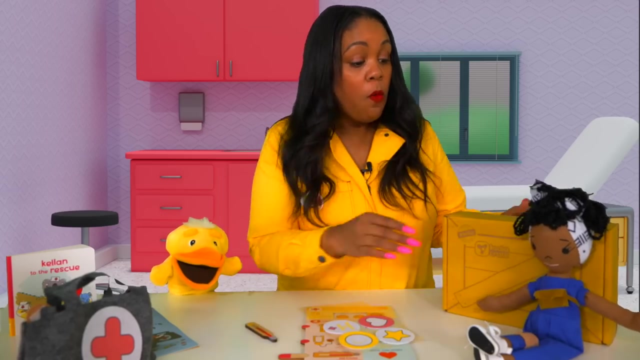 tuk, Oh, bandage. Okay, Sit down, Mia, Right here. You did such a good job. Now I want you to go home. Oh, but wait, We forgot one thing. Tuk Tuk, We have to check Mia's heart. 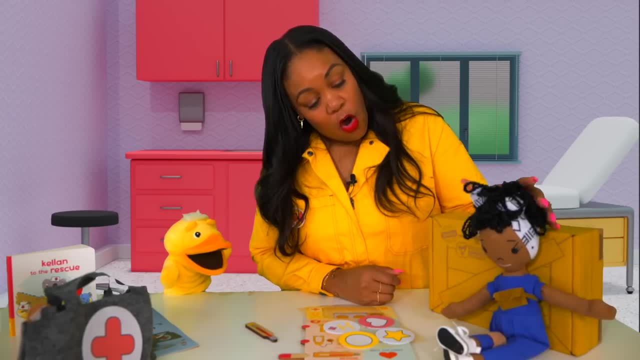 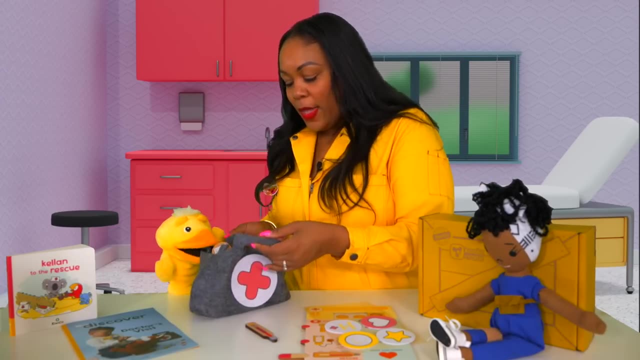 It makes your heart go fresh. Our heart is feeling okay. Can we check your heart, Mia? Yes, yes, yes, Okay, sit right here, Let's open our bag again. Thank you, that's up. Oh, look at this. 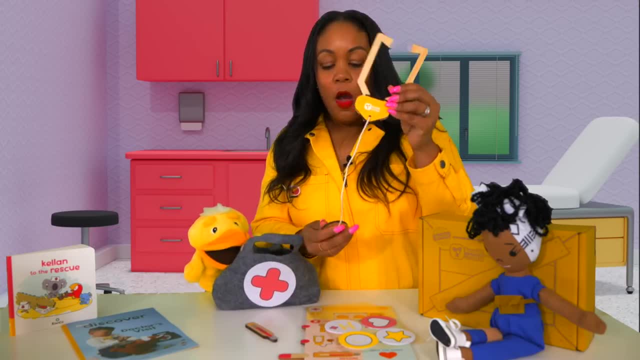 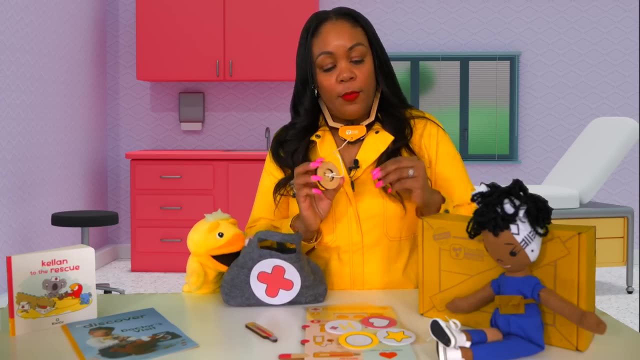 It's a stethoscope. It's a stethoscope, We can check Mia's heart. I'm going to put my stethoscope on, just like doctors do, and I'm going to put it next to Mia's heart. Come on over, Mia. 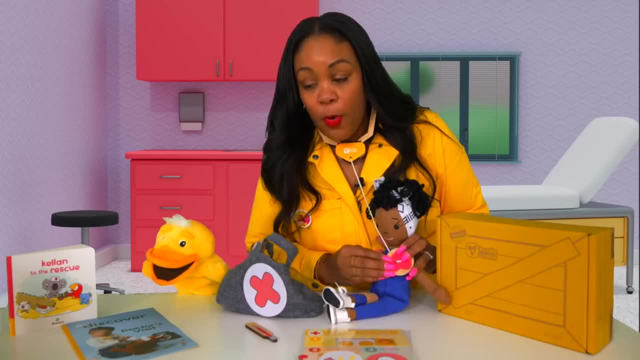 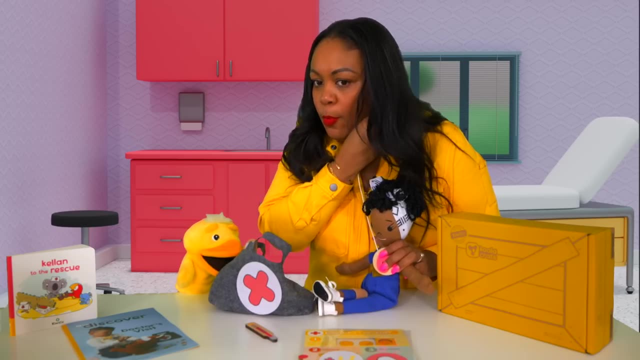 Let's help Mia sit here. Okay, Boom boom, I hear her heart, Boom boom, Let me listen. Boom boom, Oh, I can put it on my ears. Boom boom, Duck, duck. do you want to hear? 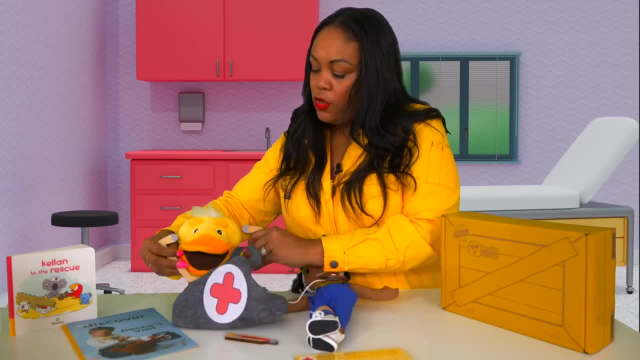 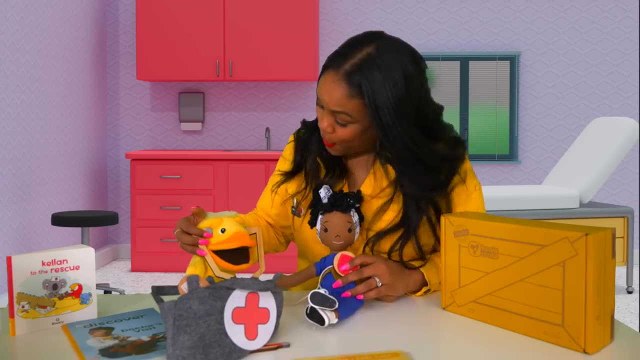 Quack, quack, quack. Okay, duck duck wants to hear too. Let's put it on your ears. duck duck, Listen to Mia's heart. Boom, boom, Boom, boom, Boom, boom. I hear it. 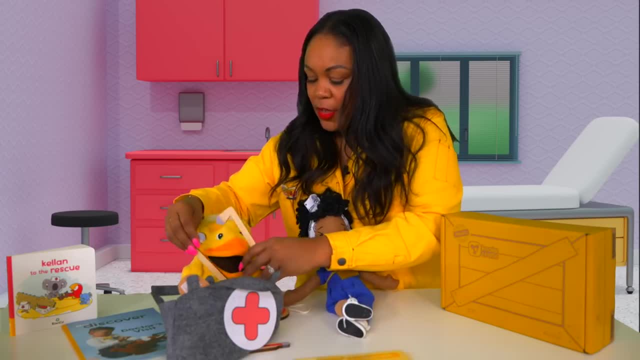 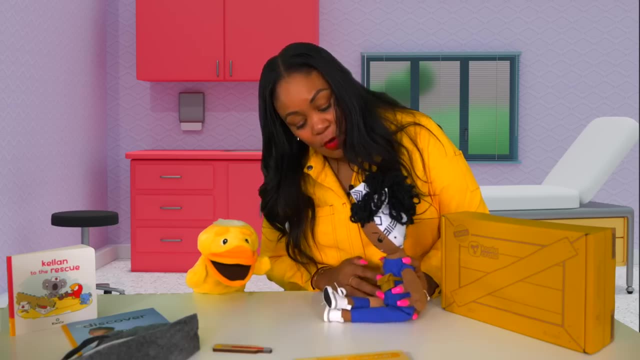 Oh, Mia, your heart sounds very good. Thank you, duck duck. Nurse, duck duck is always such a great helper. Thank you, Okay, Mia, how are you feeling now? Ah, a little better. Okay, Mia, you have to drink lots of water. 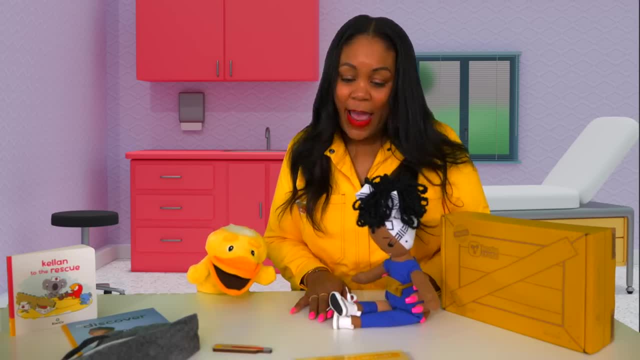 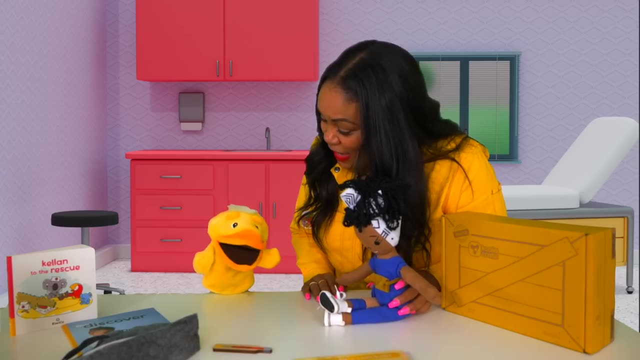 and get lots of rest and you have to go home and lay down, Take a nap, Okay, Oh, but you get a sticker. You did such a good job. Should we give Mia a sticker? duck, duck, Quack, quack, quack. 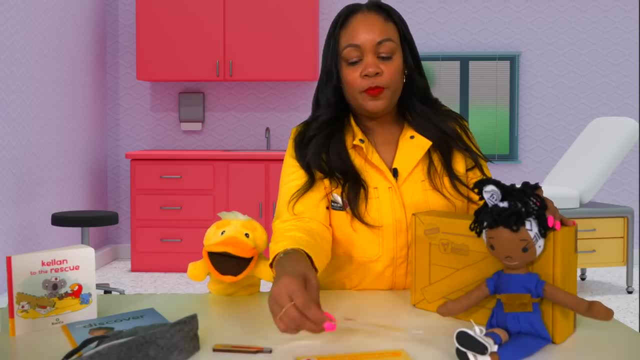 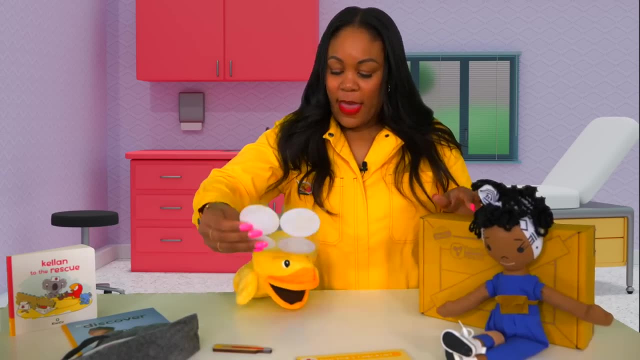 Yes, we should. Okay, let's give you a sticker. Do you want a smiley face or a heart? Ah, a smiley face for Mia. Okay, hold this duck duck. Can you help me? Okay, I'm going to take off the smiley face. 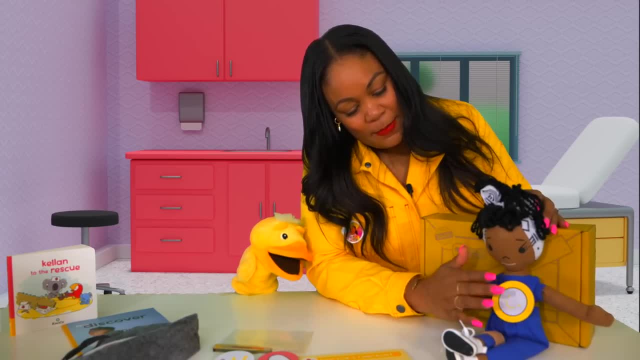 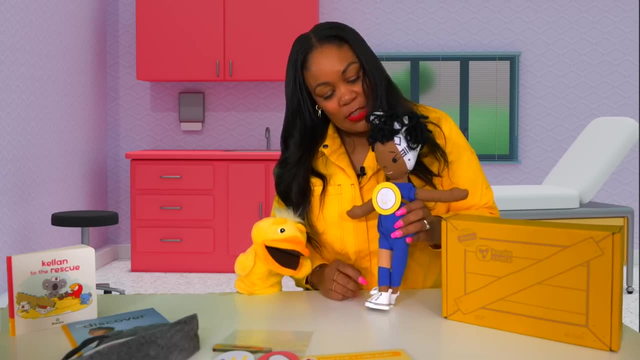 Thank you, duck duck. Here's for Mia. Tap, tap, tap, All better. Yay, Thank you for coming to the doctor's office. We'll see you again soon. Duck duck, say bye, Quack, quack, quack. 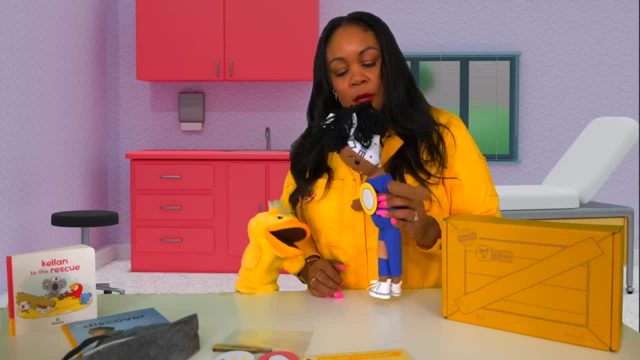 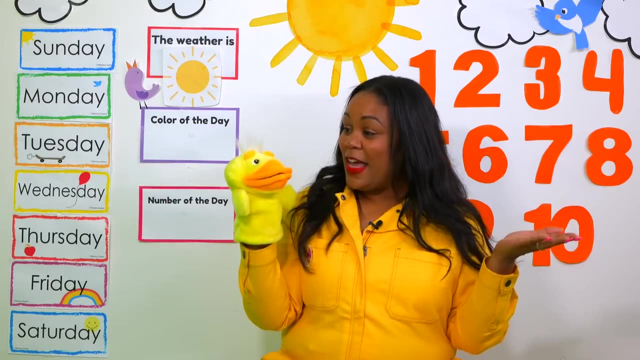 Bye Mia Quack quack quack. Bye everyone. Bye nurse duck duck. Bye Dr Monica. Bye, bye everyone. Ha ha ha ha. That was so much fun, Did you have fun, duck duck? 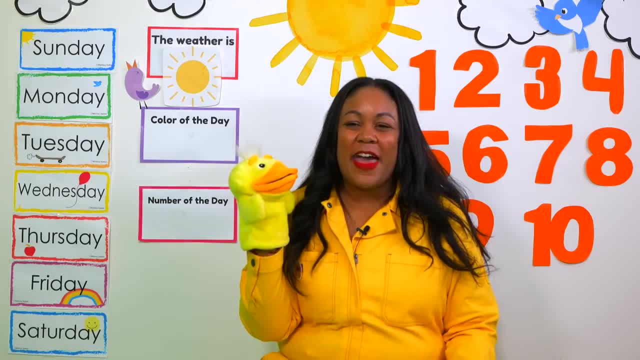 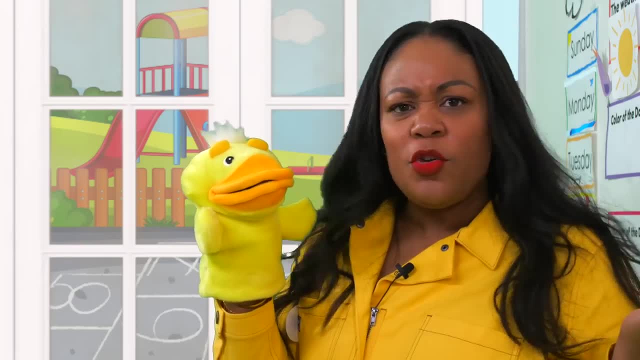 I did Quack, quack, quack. Oh, I'm so happy you had fun. Miss Monica, you look like me today. I do. Why do I look like you today? You're wearing yellow. I'm yellow too. 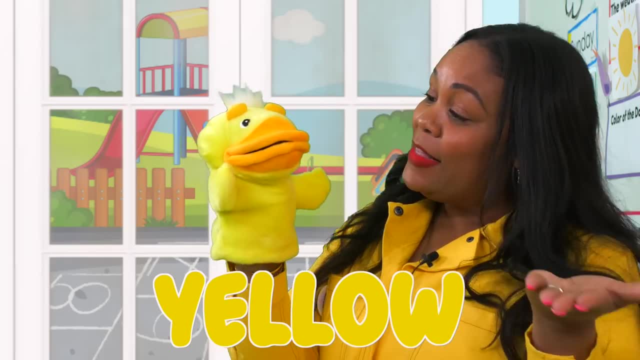 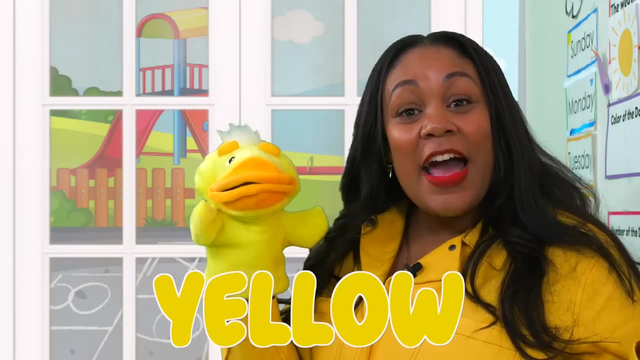 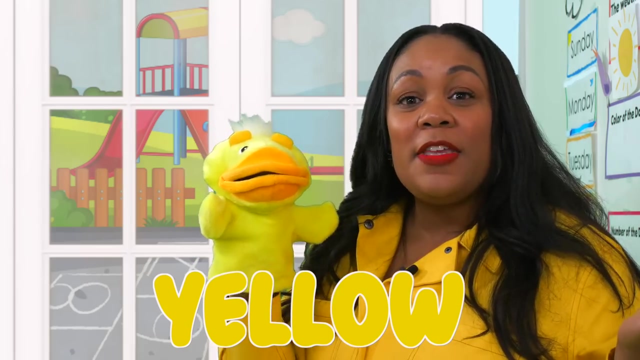 You are yellow, I have on yellow and duck duck is yellow. Can you say yellow? Good Again, say yellow, Yes, yellow is our color of the day. Oh, duck duck, how about we think about things that are yellow? 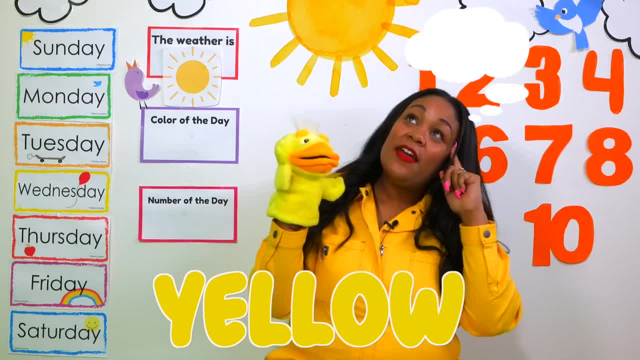 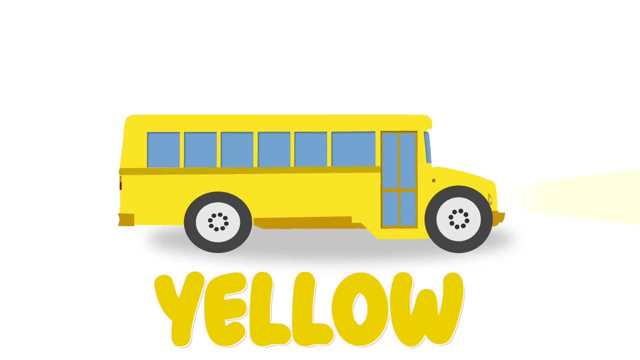 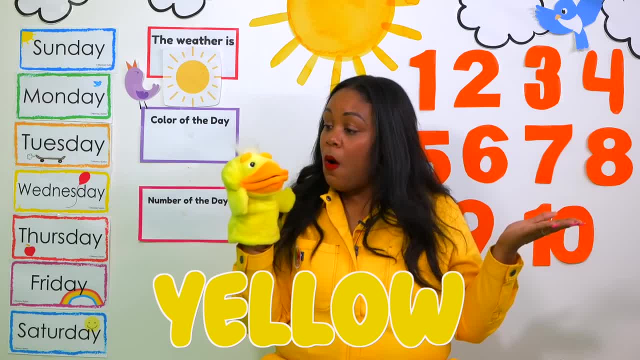 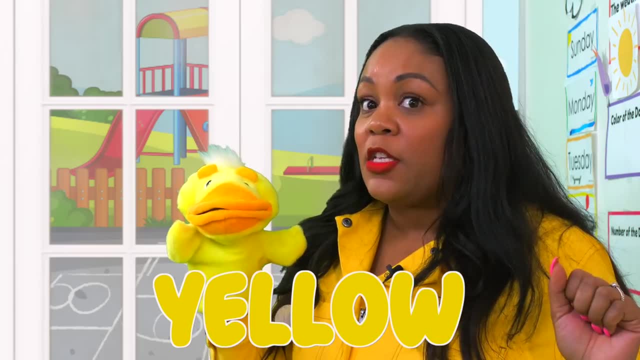 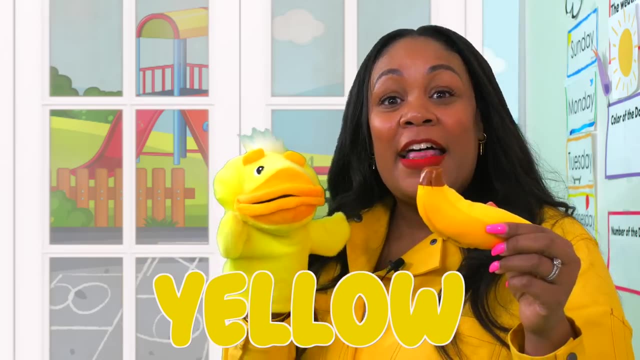 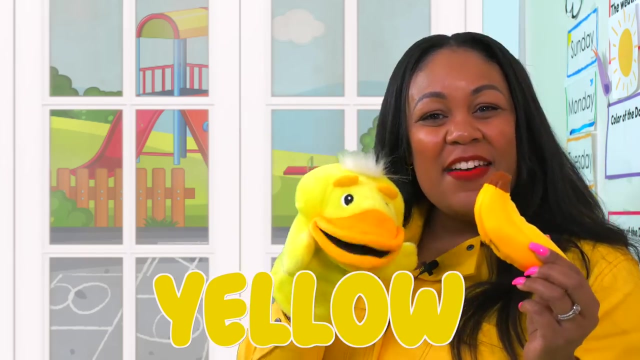 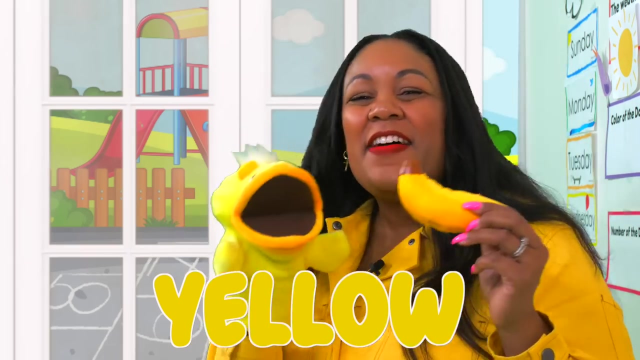 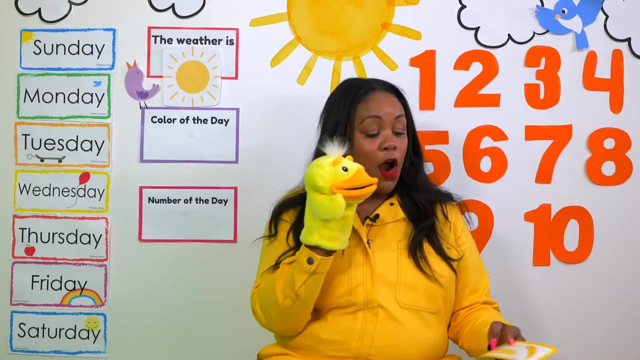 oh, can you think of anything else that's yellow? i'm thinking, oh, i think i have something that's yellow. let me look in the special box. oh, it's a yellow banana. let's sing: yellow banana, yellow banana, yellow, yellow, yellow, again yellow banana, yellow banana, yellow, yellow, yellow. a yellow banana. oh, today, our color of the day is 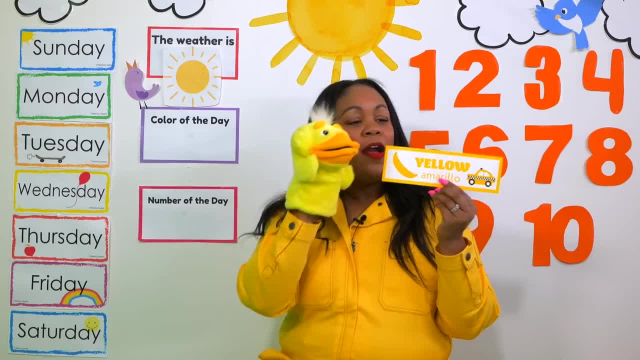 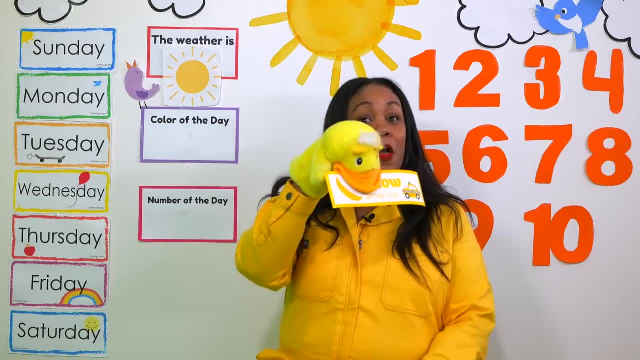 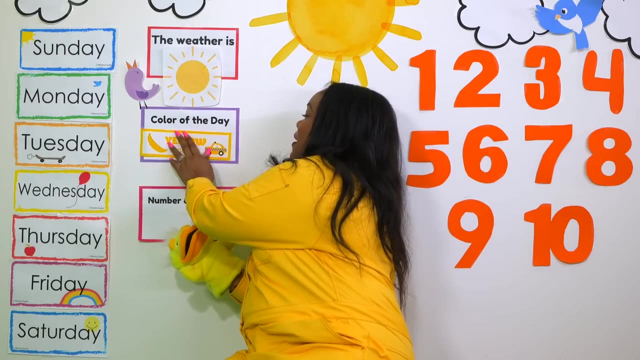 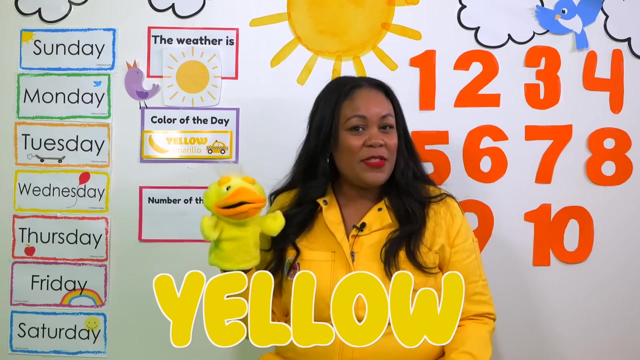 what color? duck duck? yellow. let's put yellow on the board. will you help me, duck duck? yes, i will. here we go. thank you, duck duck. okay, i'll take it from here. and top, top, top, yellow. let's say it one more time. can you say yellow, wonderful, oh, thank you, friends and thank. 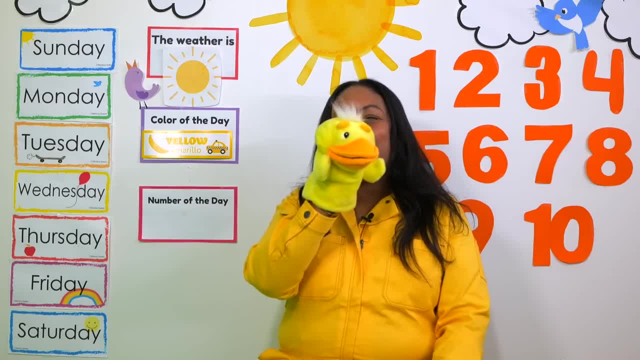 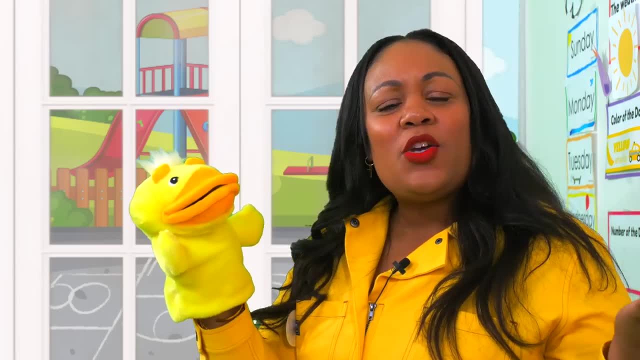 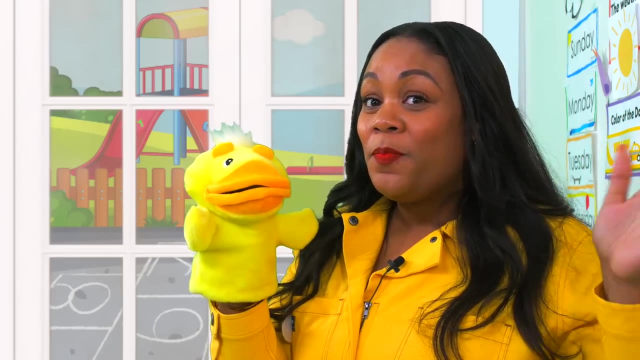 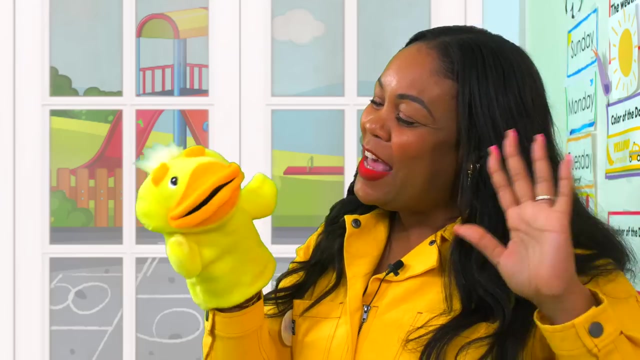 you, duck duck, for your help. you're welcome. oh, miss monica and friends, it's time for me to go. it is oh. we had such a wonderful time with you. let's say goodbye to duck duck. everyone put up your hand so we can wave: bye, bye, duck duck, bye, bye, duck duck, bye, bye, duck duck. we're so happy. 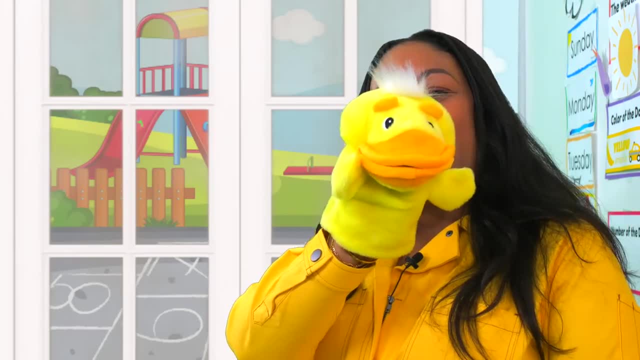 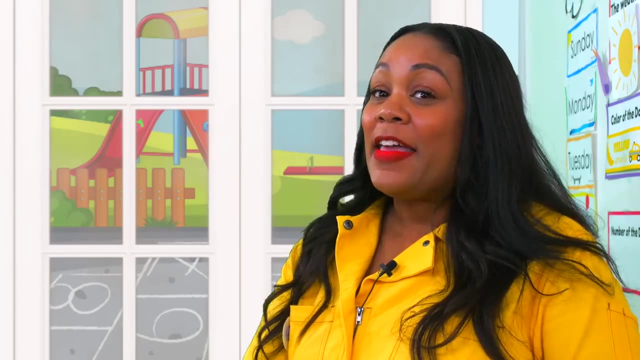 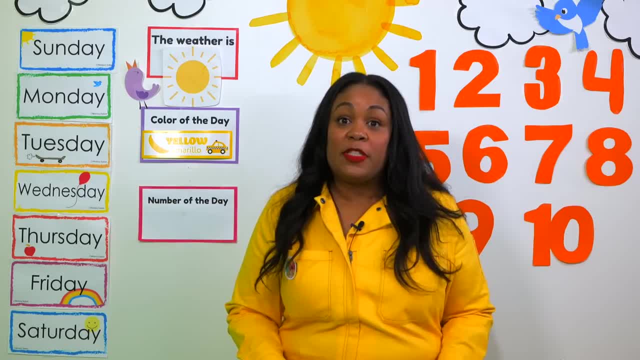 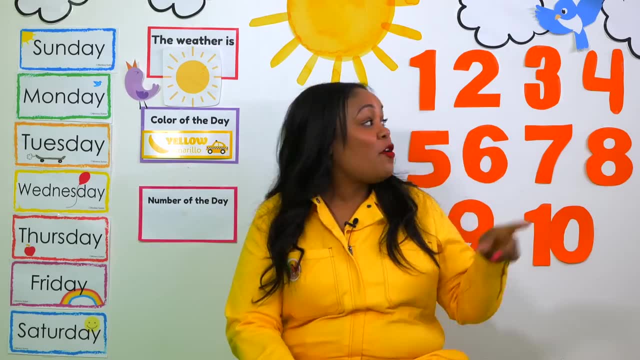 Oh, my friends, it's time for us to do some counting today. Are you ready to do counting? You are Okay. let's head to our numbers on the board. I'm going to grab my pointer. You can get your pointer too. 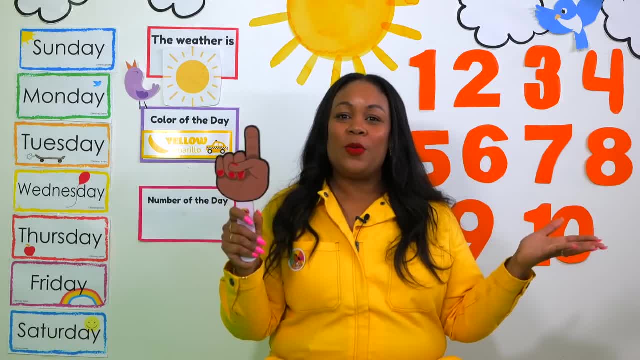 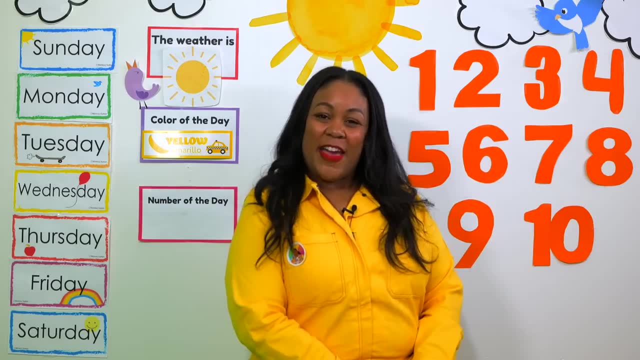 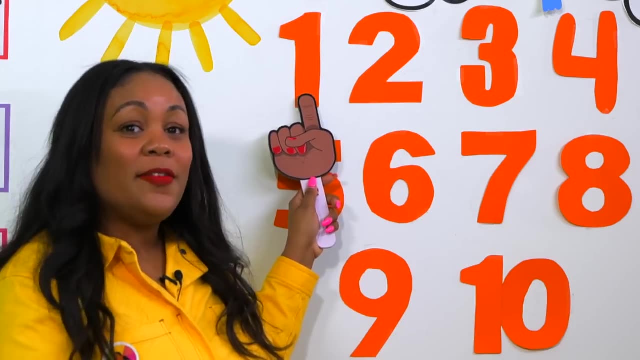 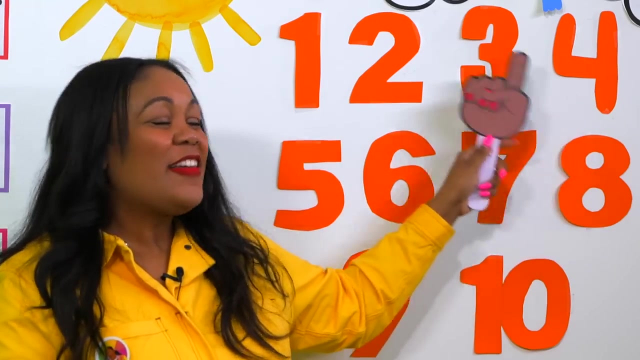 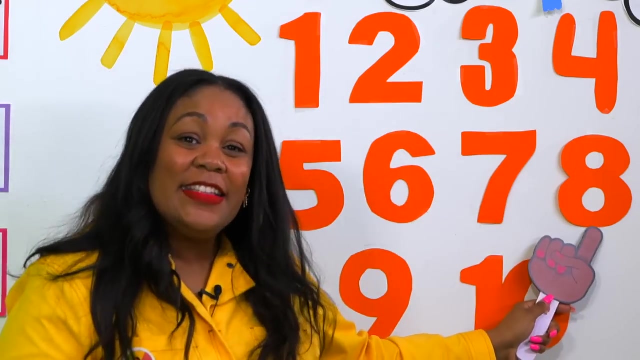 We're going to point to the numbers and count. We'll start at 1 and we'll count to 10.. Are you ready? Let's count. Let's go slow first. 1, 2, 3, 4,, 5,, 6,, 7,, 8,, 9,. 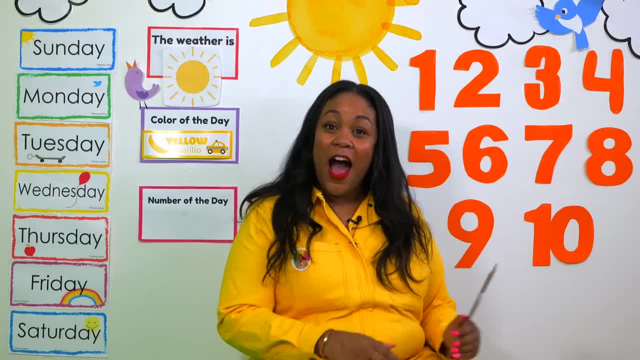 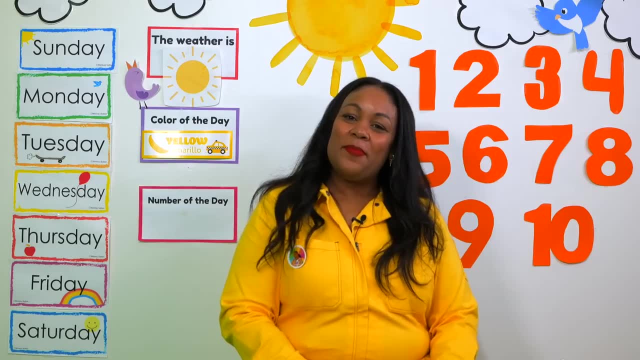 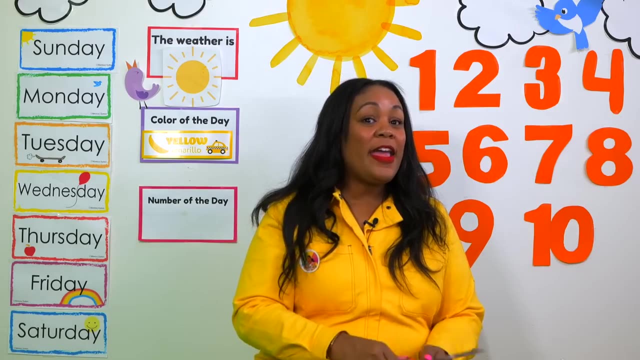 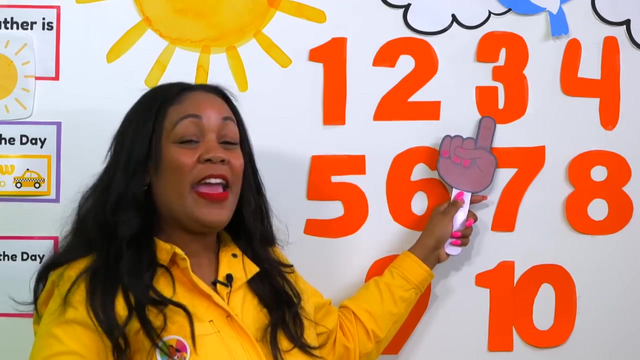 10.. You did it: Clap clap, clap, clap clap. Let's do it again. This time we'll count a little bit faster. Are you ready? Get your pointers ready, Here we go. 1,, 2,, 3,, 4,, 5,, 6,, 7,, 8,, 9,, 10.. 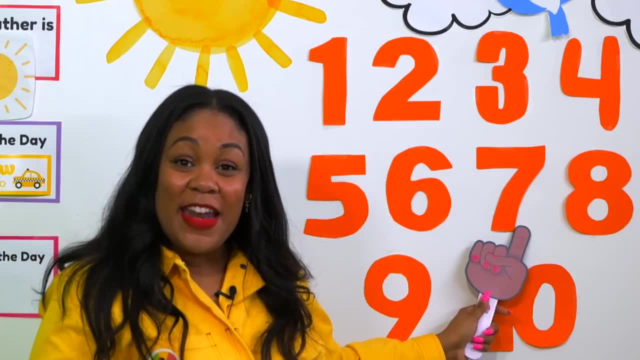 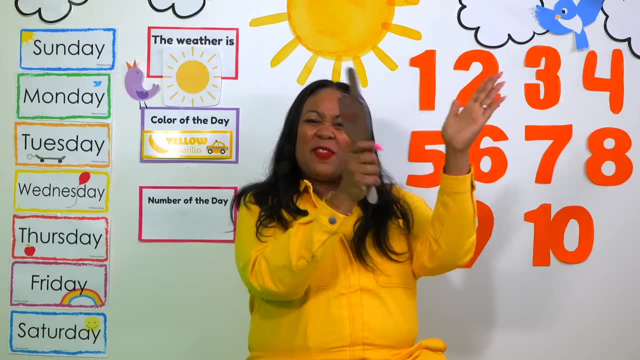 Clap clap, clap, clap clap. You did it. Oh wonderful. Oh, there's something in here. Look at this. Wow, It looks like number two. Can you say two, Two, Two, Two, Two. 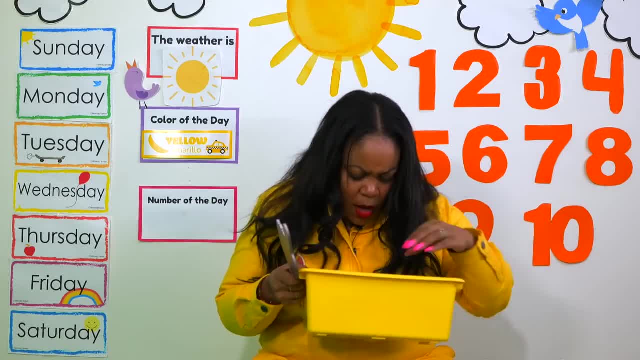 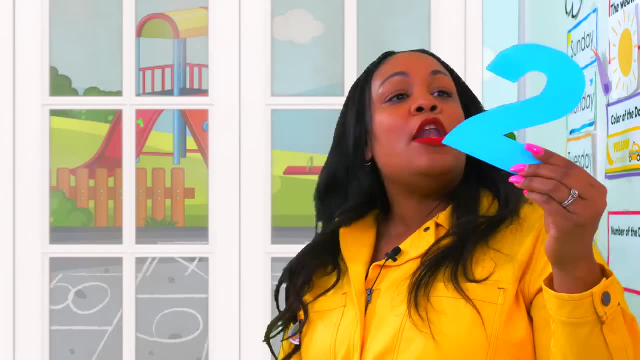 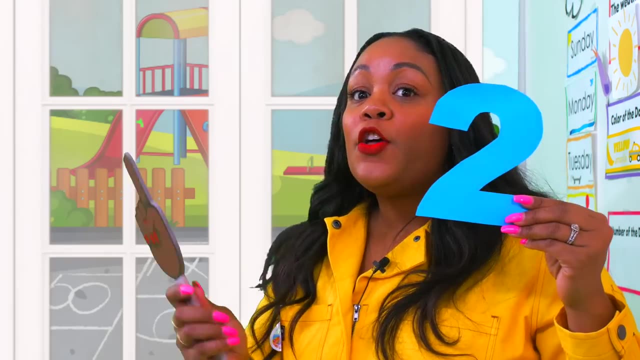 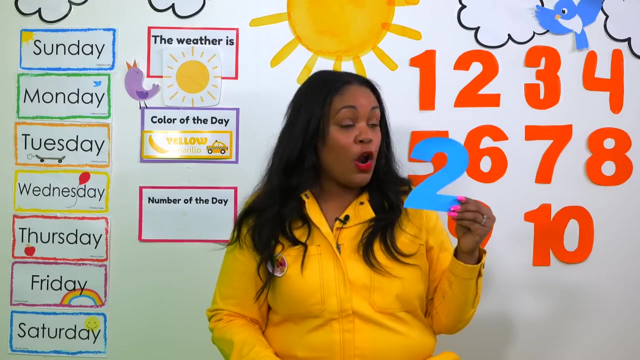 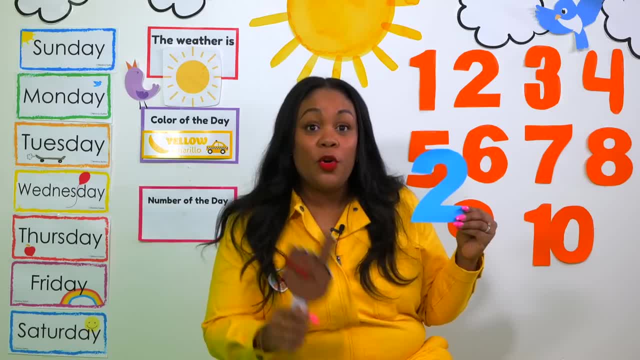 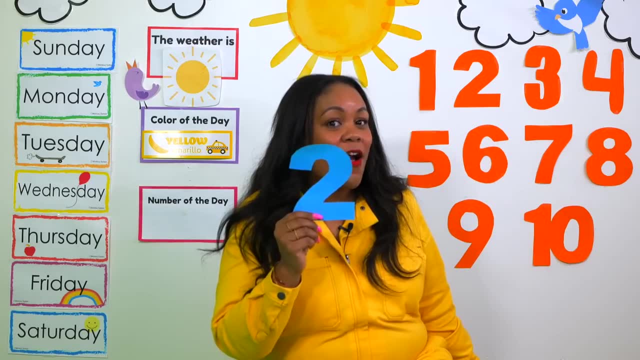 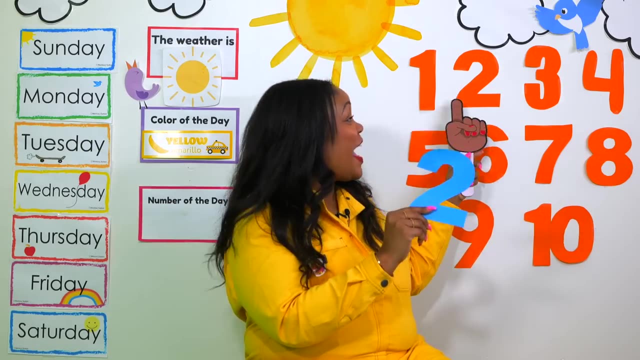 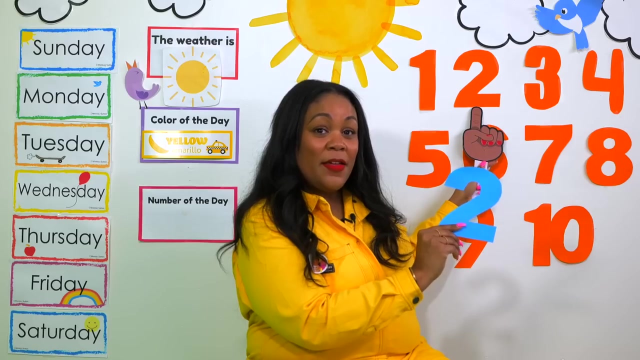 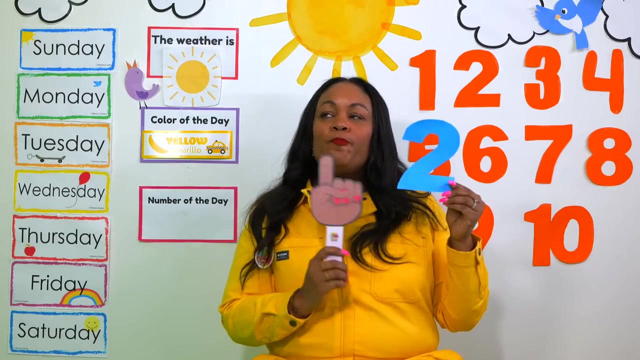 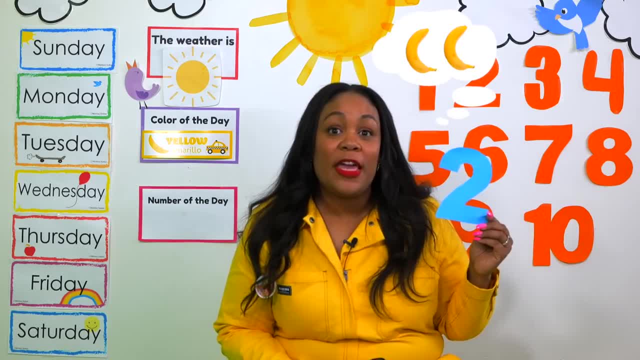 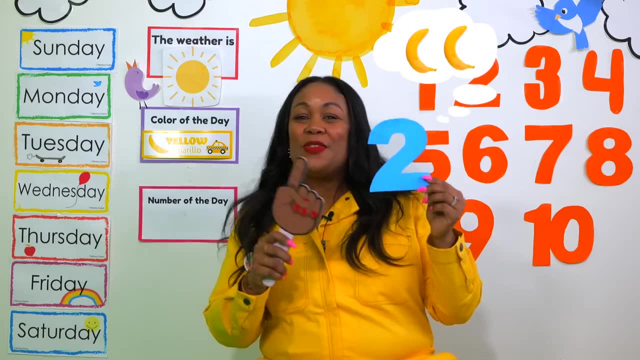 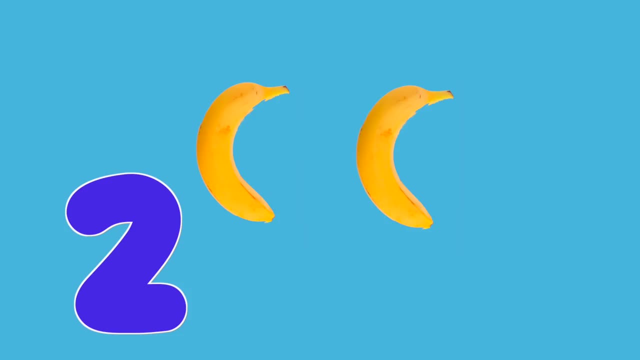 of things that have two. I can think of two things like two bananas, two bananas, two, two, two. Let's sing it again: Two bananas, two bananas, two, two, two. Let's count those bananas: One, two. 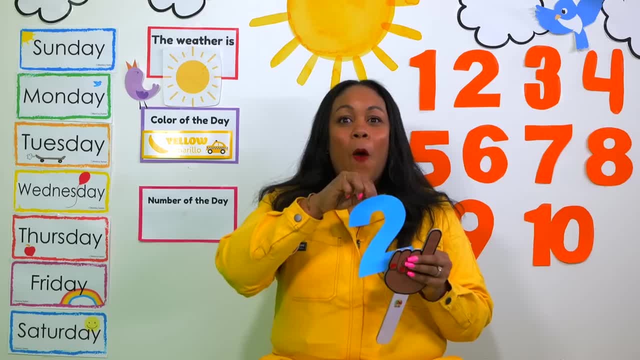 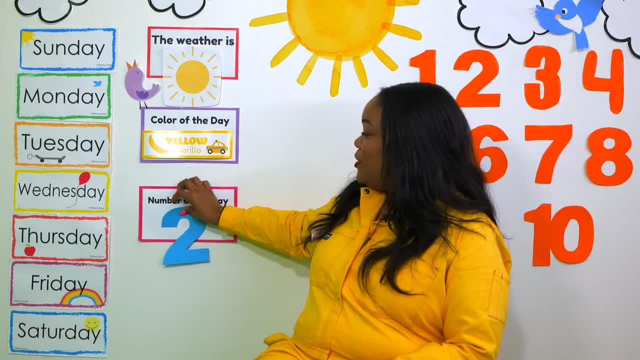 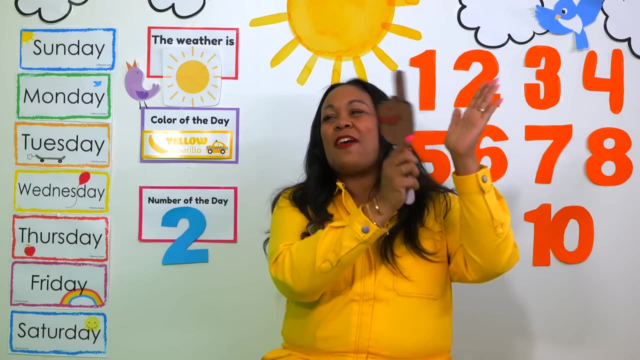 Two bananas, That's what I was thinking of. Oh, let's put two on the board. Here we go. Two is our number of the day. Two is our number of the day We did it. Clap, clap, clap, clap. 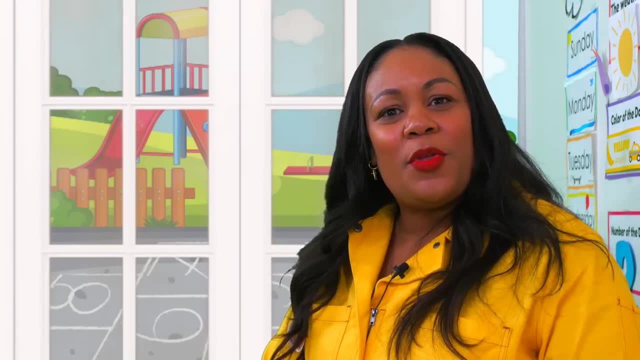 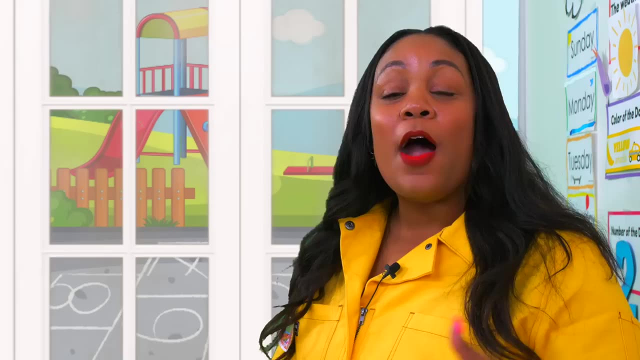 Oh, friends, I had so much fun learning with you today. Now it's time for us to sing a special song before we go. Let's sing our A, B, C's. Will you sing with me? Okay, we'll sing them. 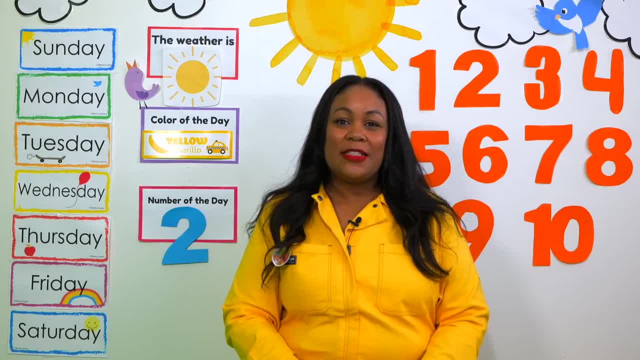 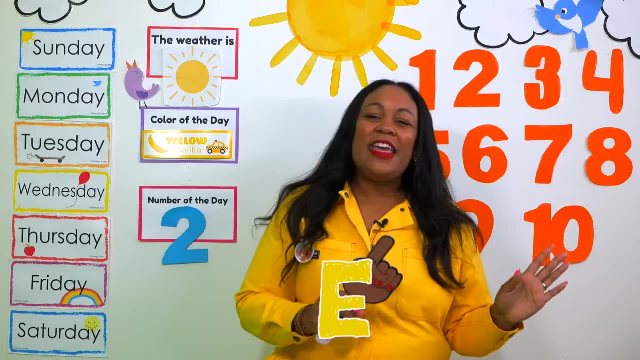 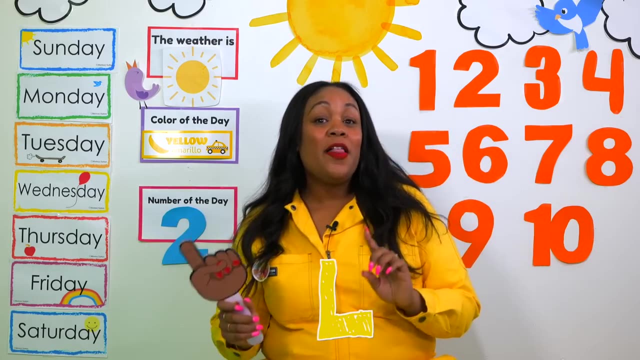 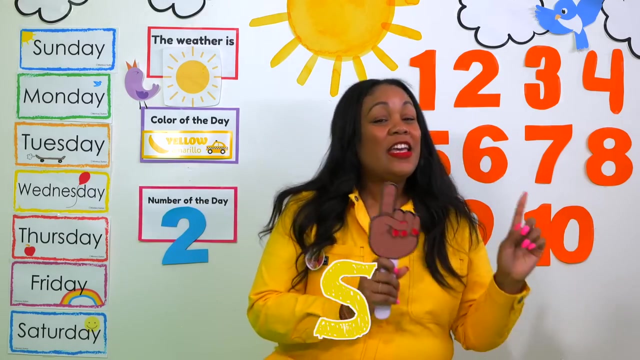 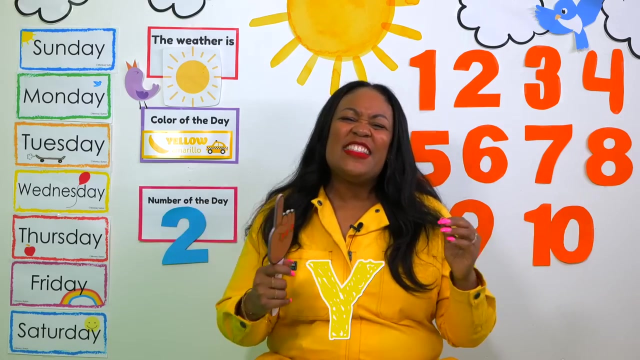 first together and then we'll sing with some of our friends. Here we go: A, B, C, D, E, F, G, H, I, J, K, L, M, N, O, P, Q, R, S, T, U, V, W, X, Y and Z. Now I know my.